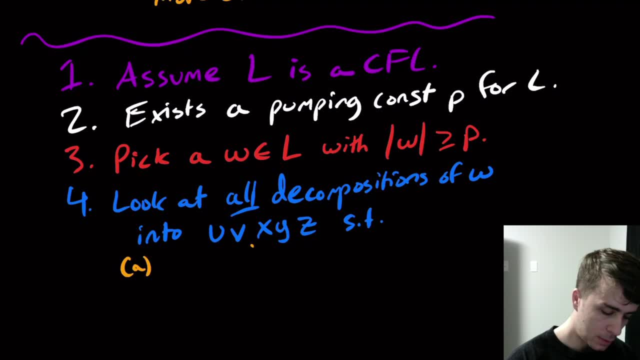 oh no, that's not the condition, excuse me. So there are two conditions and we use the third one to get the contradiction, which is the length of v, y is at least one, so one of the two is non-empty and b the length of v, x, y whole thing. 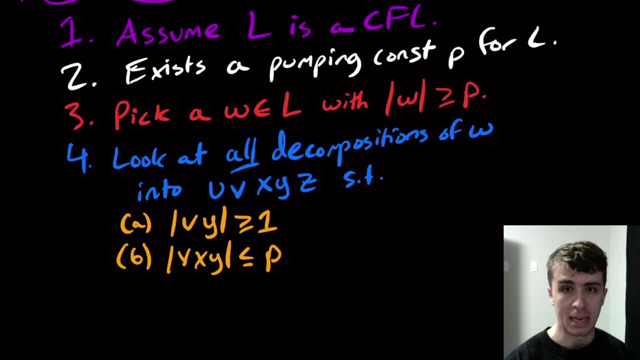 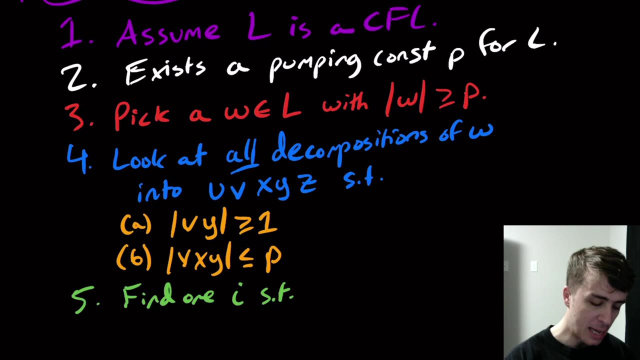 so including the x part is at most P characters. And as the final trick in my magic act I'm going to, we got to find one value of i, so find one. i such that u, v to the i, x, y to the i. 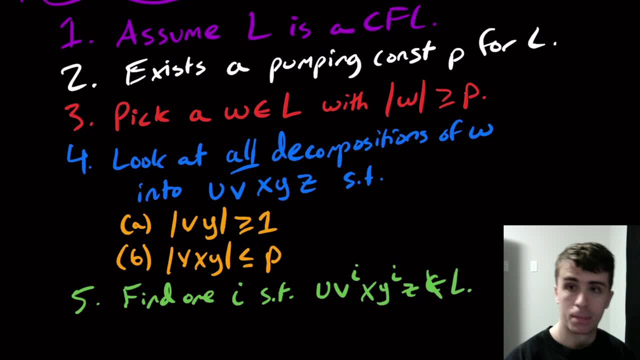 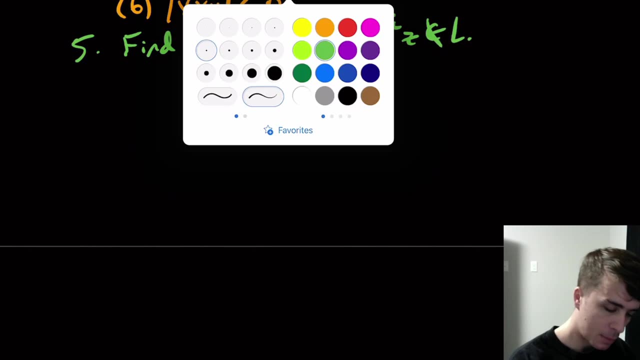 z is not in L because the pumping lemma says that it will always be in L for every choice of i. If we can find one that doesn't, then that then the language cannot have the right property, So that will show that it's not context-free. Okay, so let's do the first one, which is a to the n. 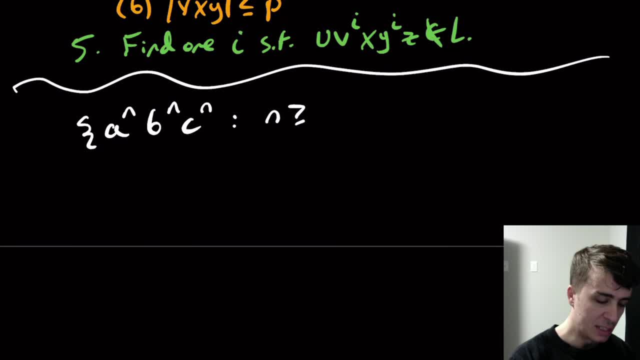 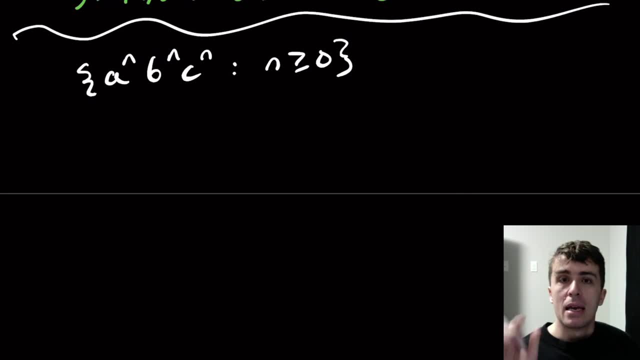 b to the n, c to the n, where n is at least zero. You would think that this might be context-free, but the intuition is, if we have, say, a PDA, for example, then the idea is: well, we push on the. 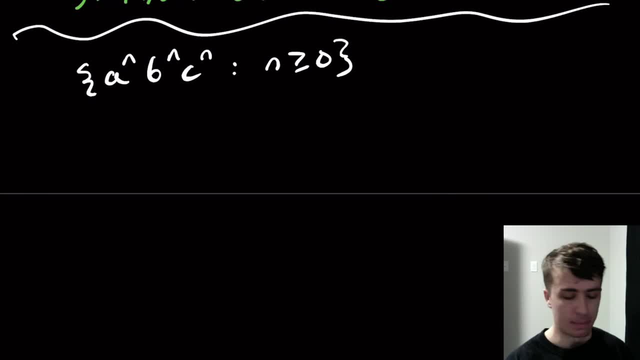 a's and then pop off the b's in tandem. The problem is that the number of c's has to match exactly the number of a's and b's individually, so they have to be exactly matching. Okay, so what do we actually do here? So, just like in my 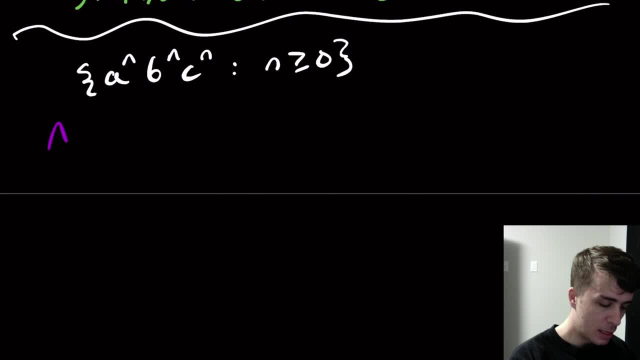 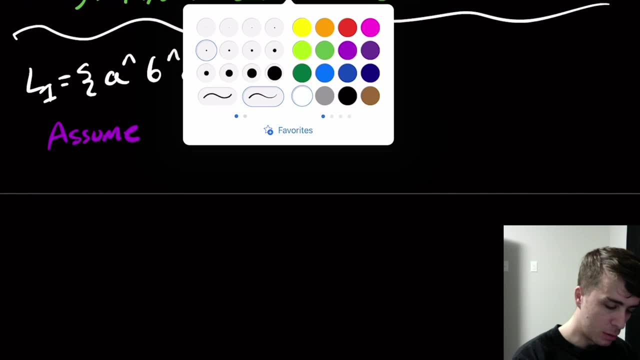 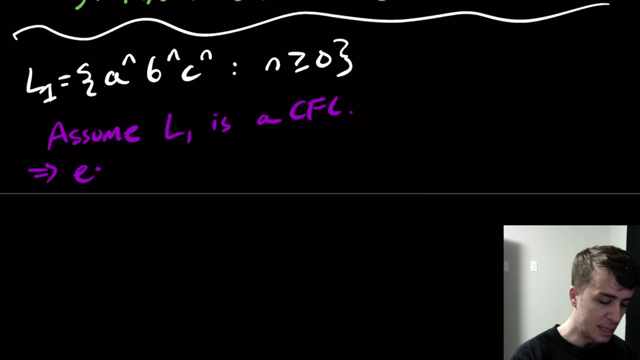 Okay, so what do we actually do here? So, just like in my, we assume: oh, I better give this language a name, so let's call it L1.. So let's assume that L1 is a CFL. Then what we know from that is that there exists a pumping. I'm only going to write it this: 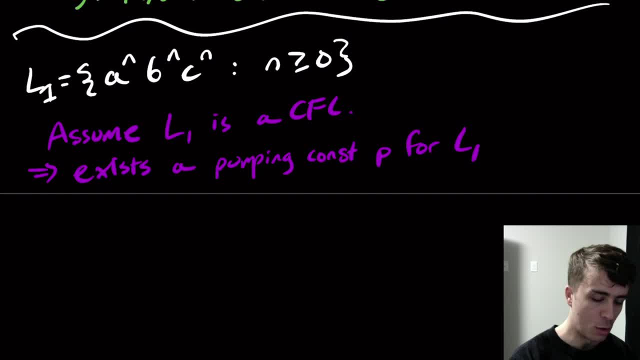 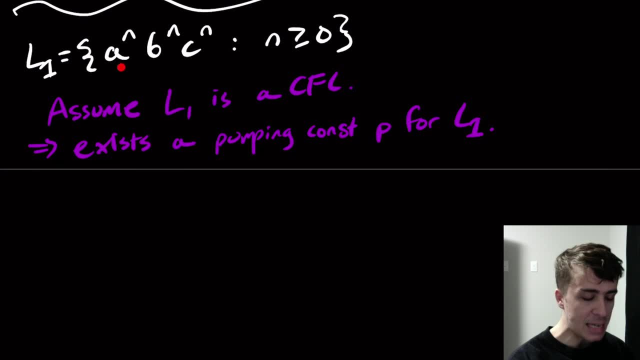 time pumping constant P4L1.. So then now we got to pick a string that's in the language, So it has an A's, followed by B's, followed by C's, and the same number of each, And it has to have length at. 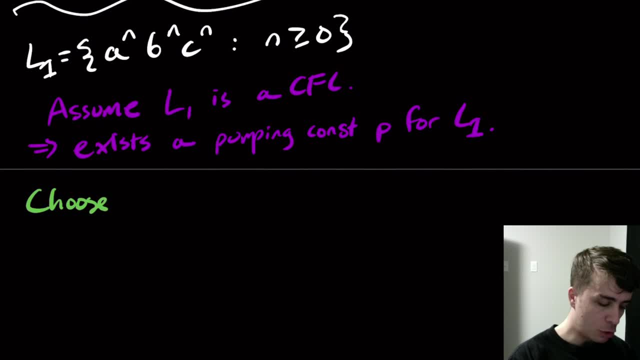 least P. So one thing that you might try is to pick A to the P over 3, B to the P over 3, C to the P over 3.. Well, that has length, at least P. There are several problems with it, But one thing is that P might not be a multiple of 3,. 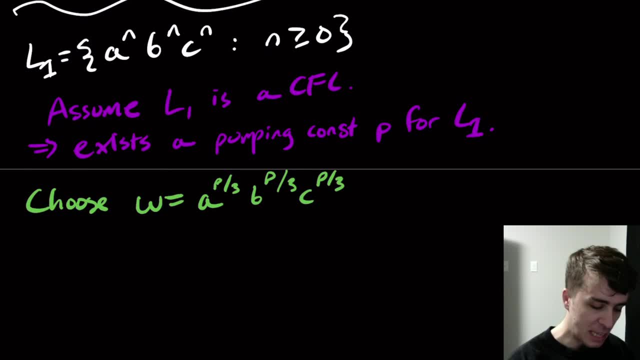 so this is not an integer, But you can fix that by, say, taking the ceiling of these if you wanted to, And that has length, at least P. But there's an easier one to write down and to actually consider which is A to the P, B to the P, C to the P. It's actually better because remember the. VXY part is the length of the string. So if you want to write down the length of the string, you can write down the length of the string. So if you want to write down the length of the string, you can write down the length of the string. you can write down the length of the string. 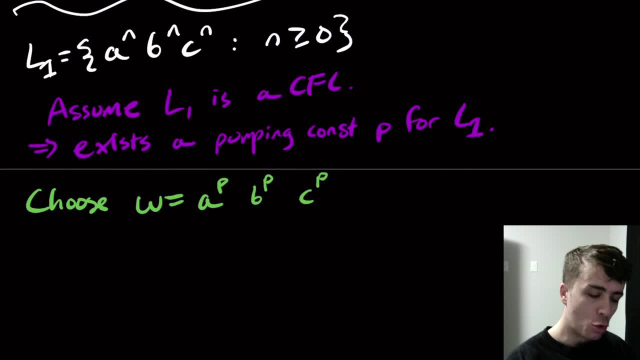 could have length P. exactly. The reason why we do that, why we do this instead, is that the VXY part, which is all consecutive, can either be in the A part or the B part or the C part, because it can technically be anywhere in the string. It can touch the A's and the B's simultaneously. It can. 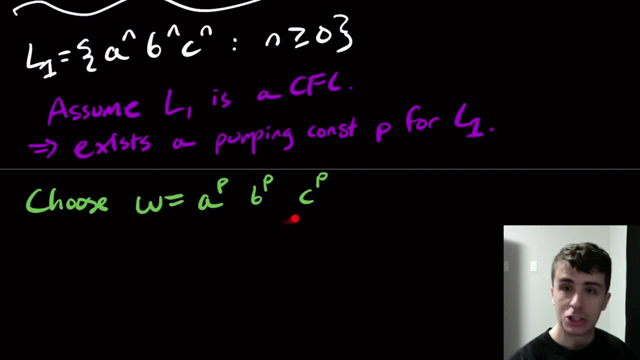 straddle between the A's and the B's, or it can straddle between the B's and the C's, but it can't hit the A's, B's and C's, So it can't hit the A's, B's and C's, So you can't hit the A's- B's. 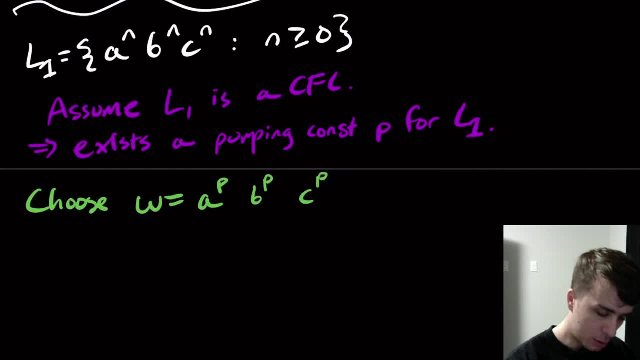 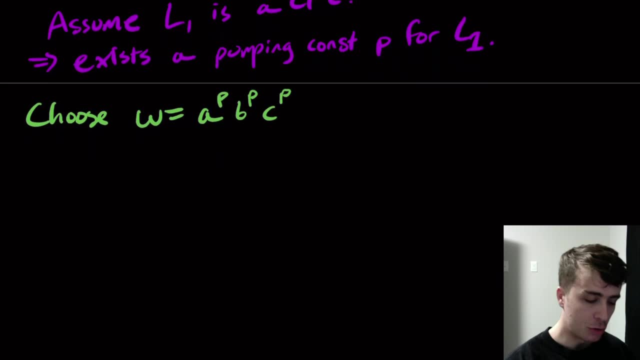 C's at the same time, which is going to be key. So let me actually make this a little more compact. So we know that this string is in the language and a length of least P. That doesn't guarantee it'll work, but it's a good starting point. 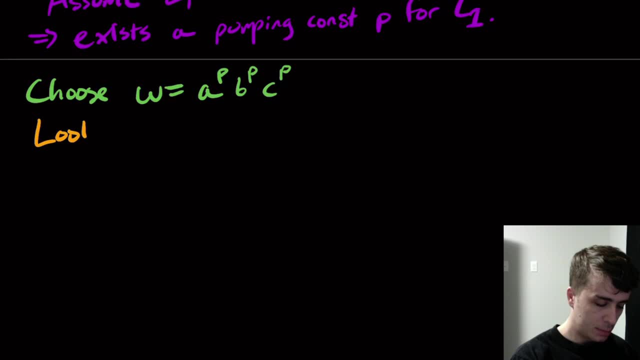 All right. so now we need to look at all decompositions. So look at all decompositions. So what's going to happen when we write a new variable into those five pieces, u, v, x, y, z? Well, I don't know. according to the rules, I should say: 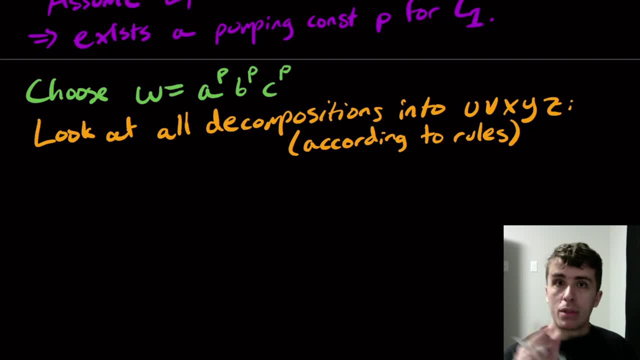 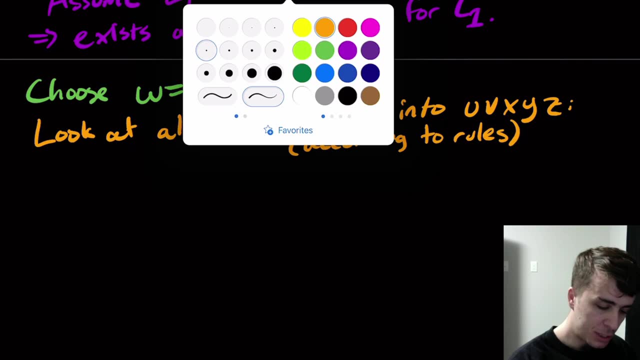 And I'll only write it this time, according to rules. Well, we know that the v, x, y part doesn't have to be at the beginning. It could be anywhere, So let's see. Suppose that. So let's look at a particular set of cases. 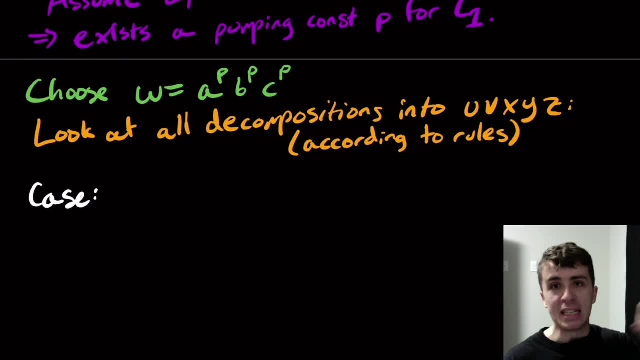 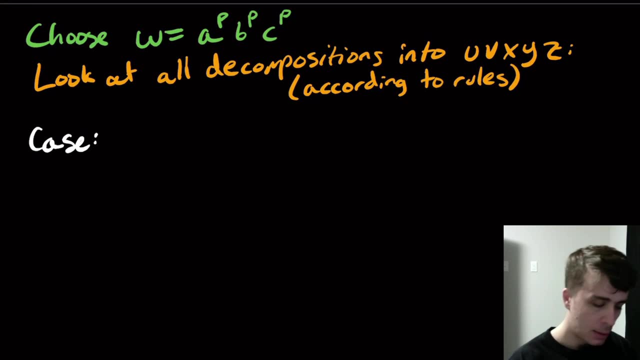 So let's say that we're going to write a new variable into some set of characters. v is equal to this, x is equal to this, because it's just not necessary And it's just going to complicate things way too much. 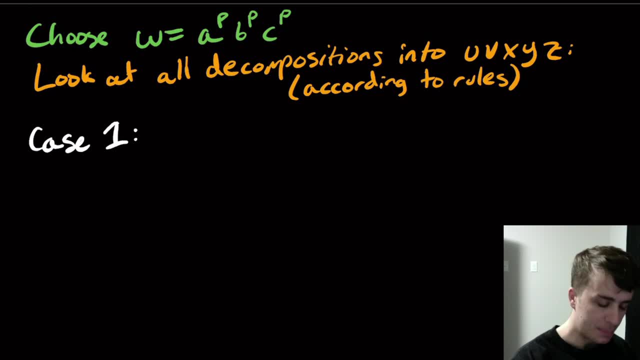 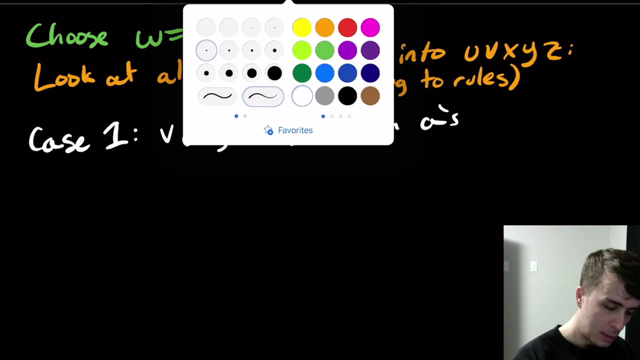 So let's look at- I'm going to call it- case one, which is that v and y are Actually- I'll write it this way- v and y only contain a's, So if we look at what the string looks like, 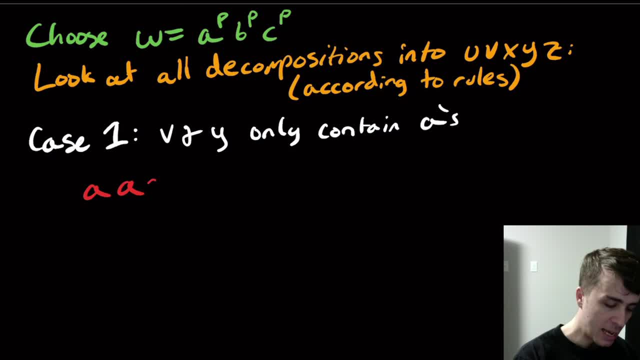 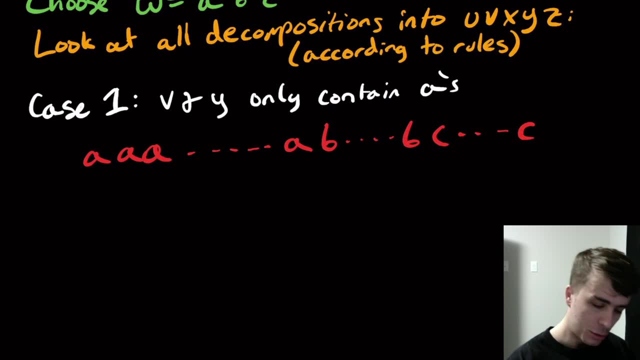 actually I'll change this to red. So we have a bunch of a's, then b's, then c's, like this. So if v and y only contain a's, then that means that the v part is somewhere in here. 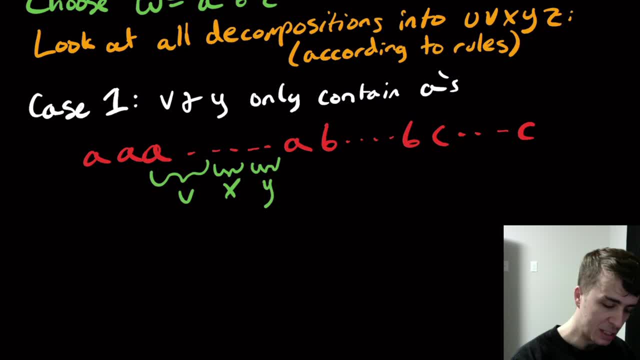 The x part is in here, The y part is in here. God, that was terrible. There, that's a little better. The z part is the rest And the u part is at the beginning. That's just what this case is saying. 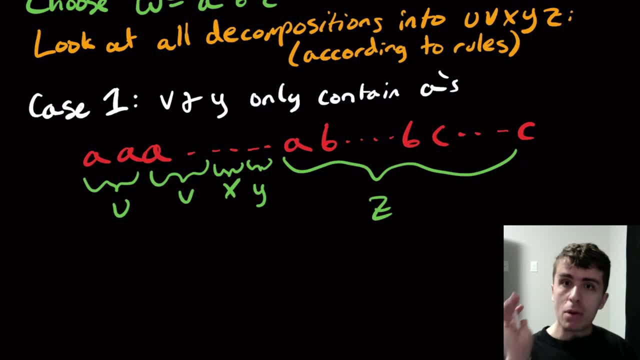 There are obviously other cases. So if we pump up, if we insert another copy of v and y in- I don't know whether v or y is not empty, but I know one of them is. So if we pump up to, let's just say, i equal two. 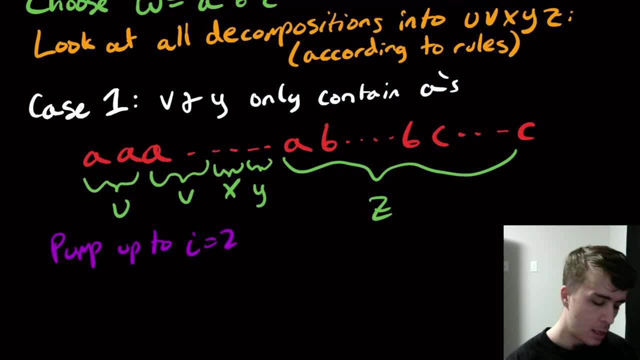 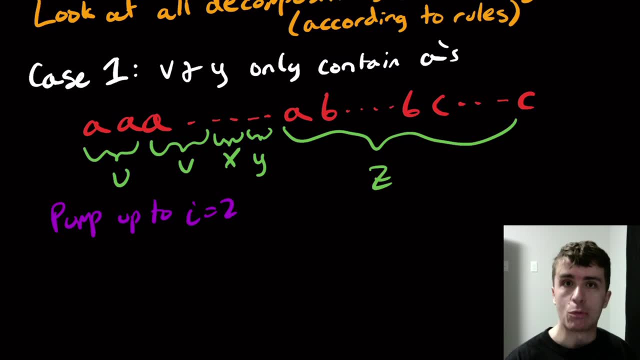 any value of i actually other than zero works here, then what will happen is that we will have more a's than we started with, because one of these two is not empty, And so we're gonna be putting more a's into the string. 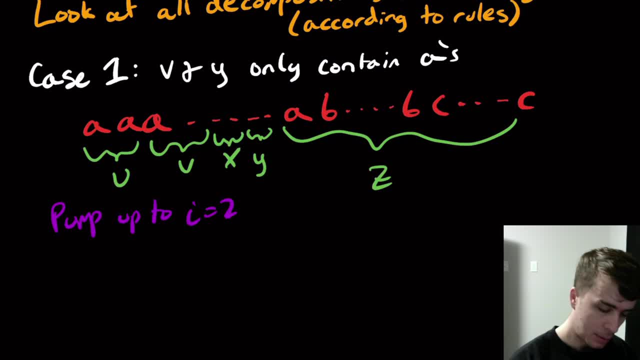 but we're not gonna be adding more b's or c's. So then this tells us that the resulting thing, which is two copies of v and y, because we're putting another copy in- has has more a's than b's or c's. 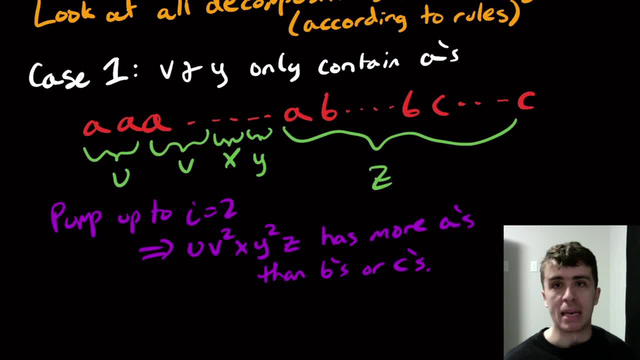 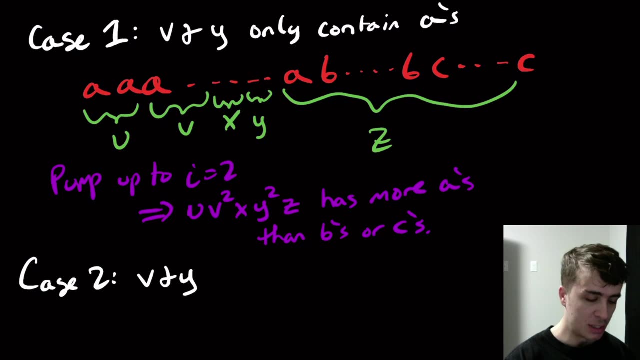 And that automatically disqualifies it from being in the language right, Because the language has exactly the same number of a's, b's and c's. All right. What if we had a different case two, And this is actually multiple cases at once. 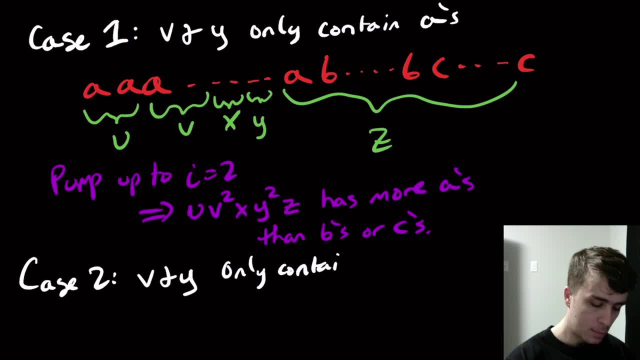 v and y only contain b's or only contain c's? Well, actually the same logic will apply, It's just the conclusion's a little different, but the same contradiction is reached. Because if they're only say, within the b part, 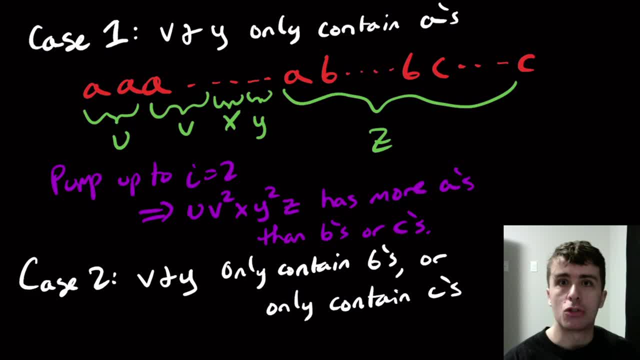 then by pumping up, we're putting more b's into the string, which means and no a's, no c's. So therefore we have more b's in that case in that case than a's or c's. and if it was only within the c part over here, then if we put more 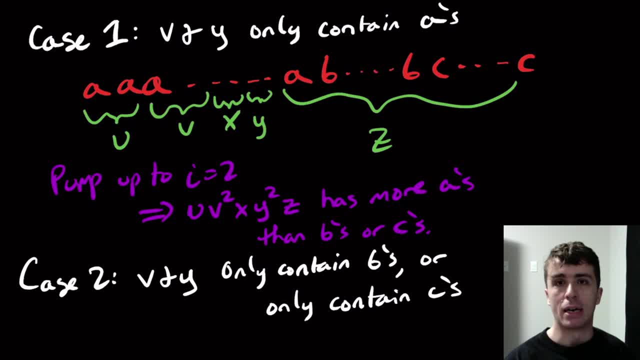 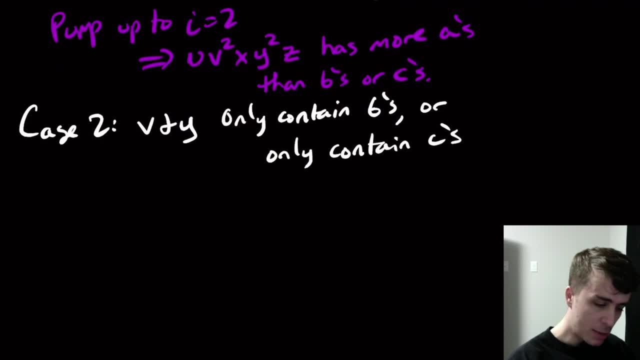 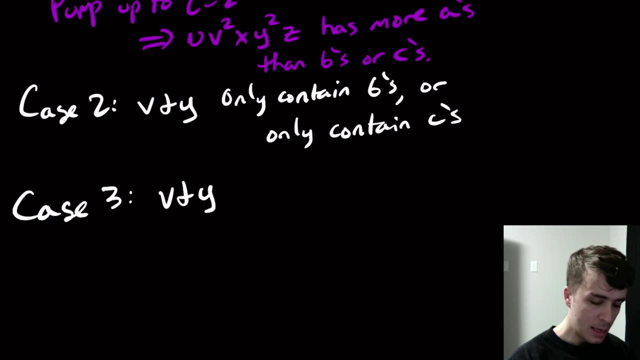 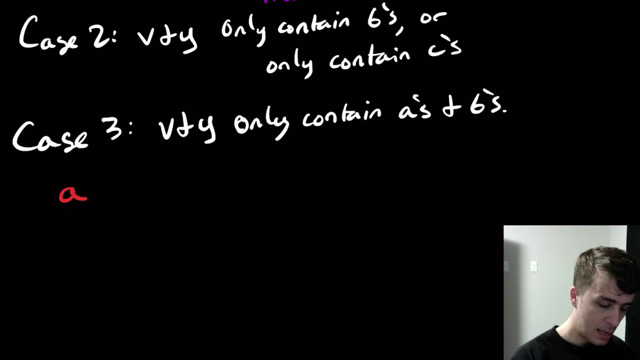 a's into the string. sorry, more seasons. this string. we're not going to insert any a's or b's, and so it's not in the language anymore. so what about the other possibility, which is case three, that v and y only contain a's and b's? so let's visualize what this looks like. so if I have a bunch of a's here, 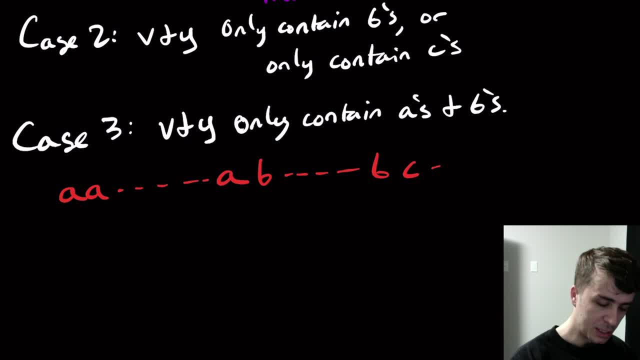 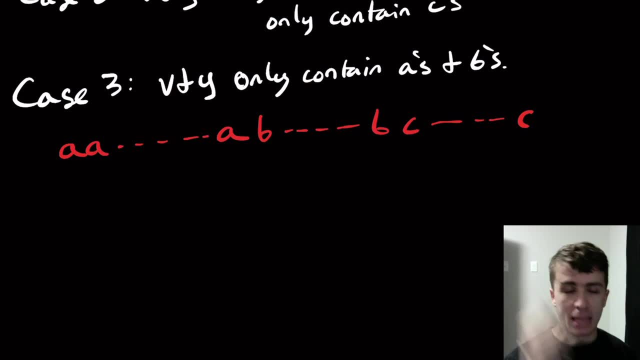 b and c. actually, you can show that in this case both of these have to be non-empty, if we weren't in the other cases. but that's not important. so the v part is over here because it's before the y part, although that doesn't matter. The x part. 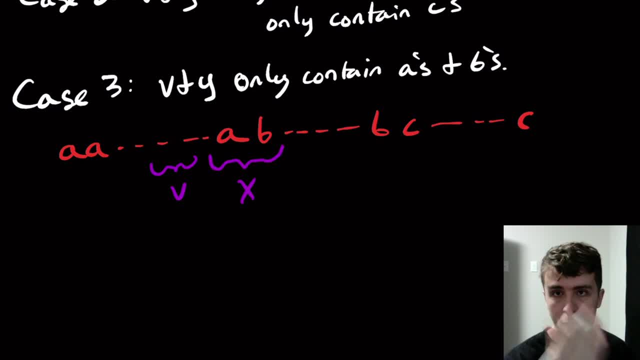 is going to be somewhere here. It may cross into the b's, We don't know for sure. But I know that the y part is in the b's only And I know this because that's what I assumed. And, of course, 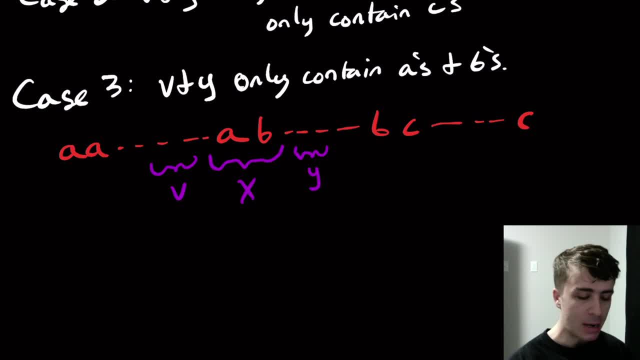 v, x, y together can be at most p characters, And each of these ranges has exactly p characters. So it can't be the case that we touch one of the a's and one of the c's at the same time, because it has to cross this gap of p characters and it can't have more than p characters. 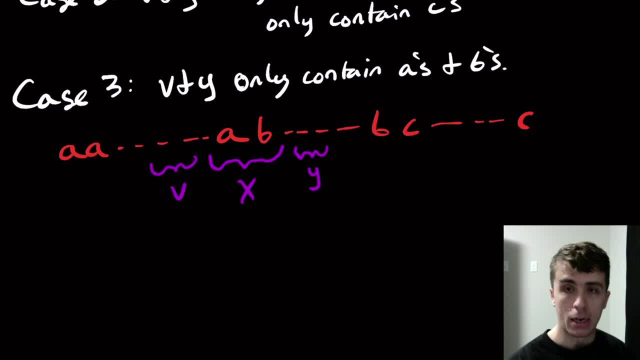 So the v part. I'm assuming here y is over here. So if I pump up again in this case, then I'm going to be putting more a's into the string, more b's into the string, Maybe the same number, we don't know- But the number of c's is not touched. 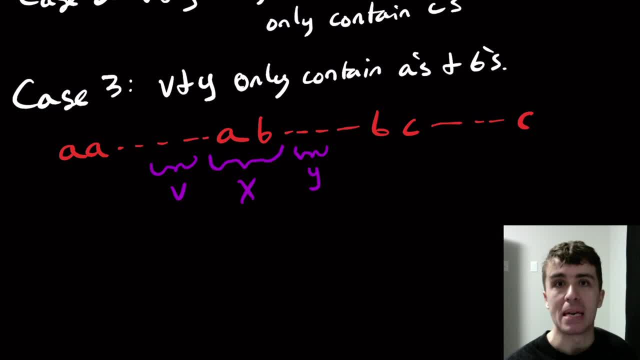 And so that's the problem. The number of a's, b's and c's cannot be the same. This actually shows right here: if we just ignore the c's and just only have a's and b's, we show that this is context-free. 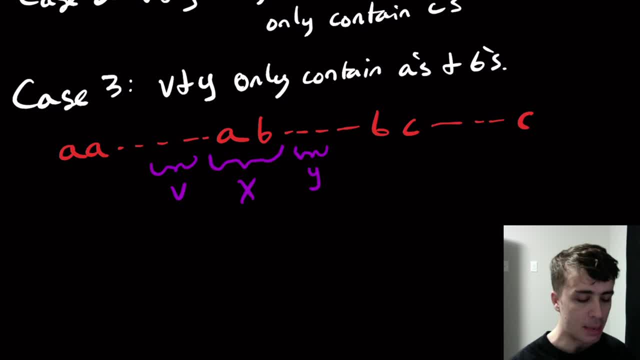 Because this decomposition: if I have the same number of a's and b's for the v and the y part, here we can actually pump up and still have the number of a's and b's. But because of these c's over here, that allows us to pump up and still have the number of a's and b's. 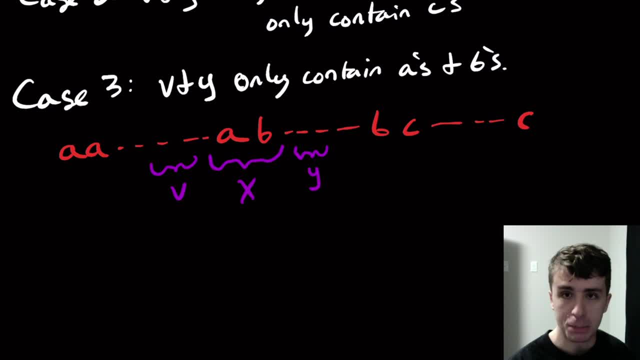 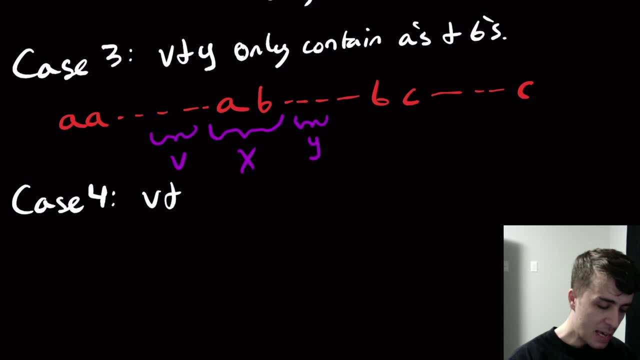 To show that this cannot be pumped in this particular case. And then if we look at the other possibility, which is that v and y only contain b's and c's- Not sure if you can hear the garbage truck out here, but the logic is exactly the same. 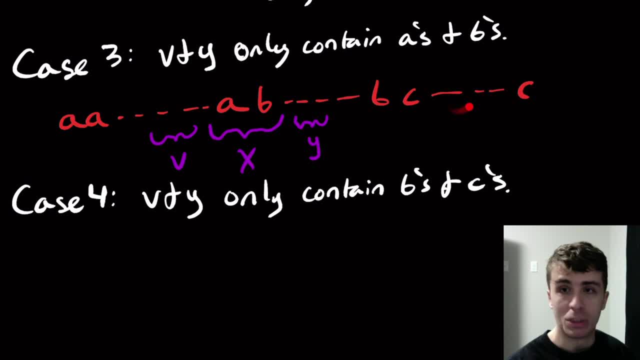 If the v part was in the b's and the y part was in the c's, then we're never, ever touching those a's at the beginning, And so the number of a's, b's and c's cannot all be the same number, And so we get exactly the same conclusion. But the important thing is: 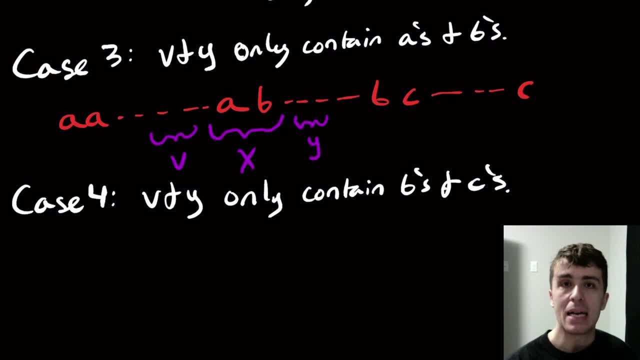 we can't have any other case because if we, the only possibility of another case being is that we have a's, b's and c's- but we just discussed that that can't possibly happen because we made these gaps so big, These consecutive parts of the string, they have p characters each. That's why I was saying p over. 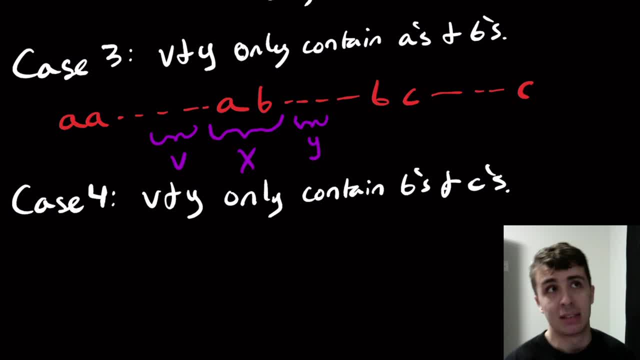 three. that idea doesn't work as well, because in that case you could have a's, b's and c's at the same time. But by making these big enough, we can show that we can actually not have to worry about that possibility, And so, because of this, in all cases, 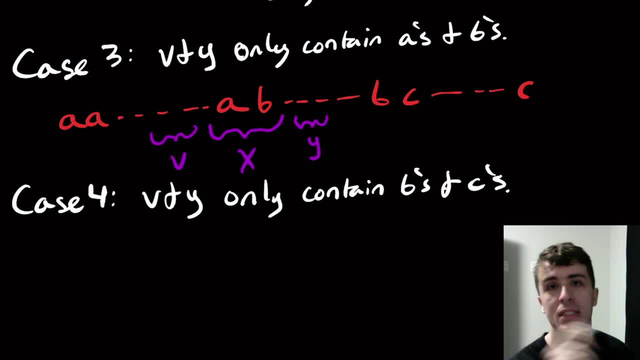 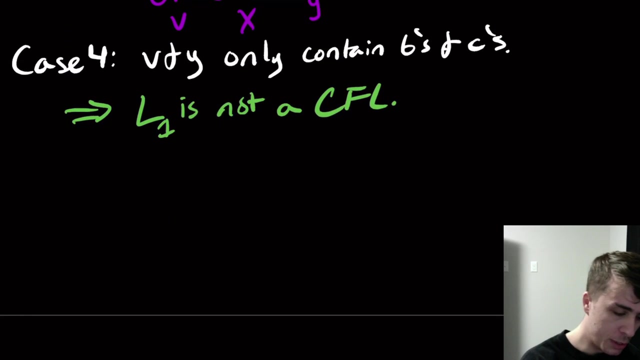 we're able to pump out of the language. We could have a- we have a different value of i, possibly at each time, and we'll see an example of this- But we were able to pump out of the language in every possible case. So that shows that that l1 is not a CFL. All right, So let's go on to the next. 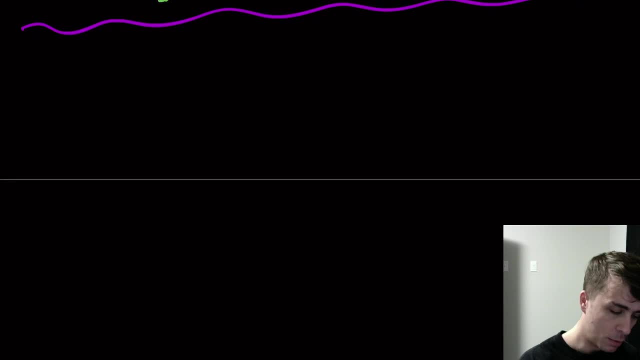 language, which is very simple, So we're going to call it l2, which is a to the i, b to the j, c to the k, where- not that they have to have the exact same exponent, but i is less than or equal to j, less than or equal to k, And actually the proof is slightly different. 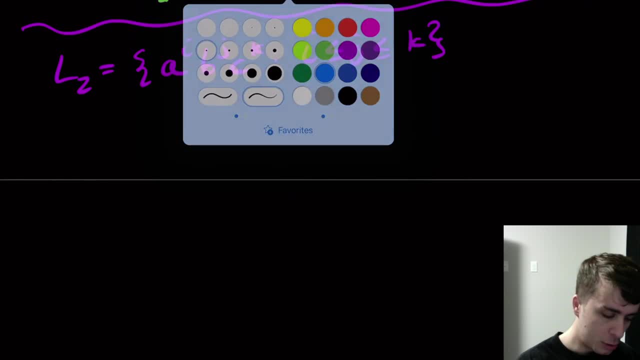 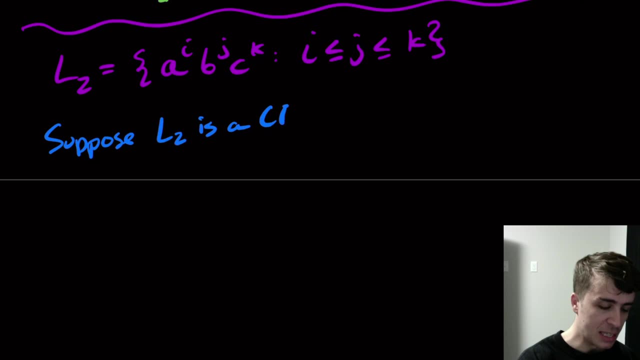 but it's very, very similar. So we got to start as usual. We're going to suppose that l2 is in fact a CFL And I'm just going to shorthand this. There exists a pumping constant p for l2, this language. 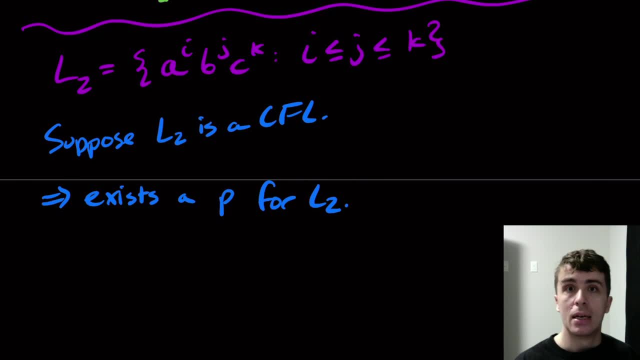 And of course, just like now, we need to pick some string that's in the language and long enough, at least p in length. So I'm actually going to choose w to be exactly the same exponent in all cases, And that's okay, because we have a less than. 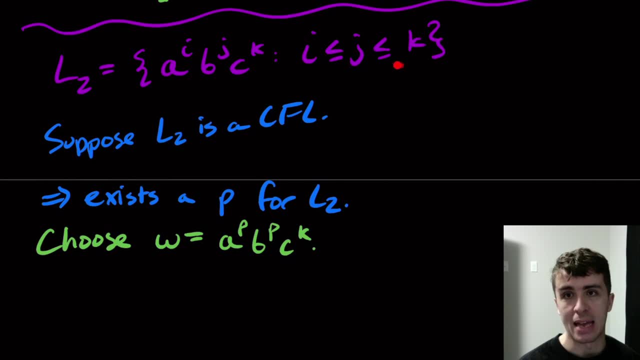 or equal to for the i and j and j and k here. Oh, I put k here. That's not what I wanted. I wanted p. And why is this a good idea? Why not put like plus one or plus two here, or whatever? 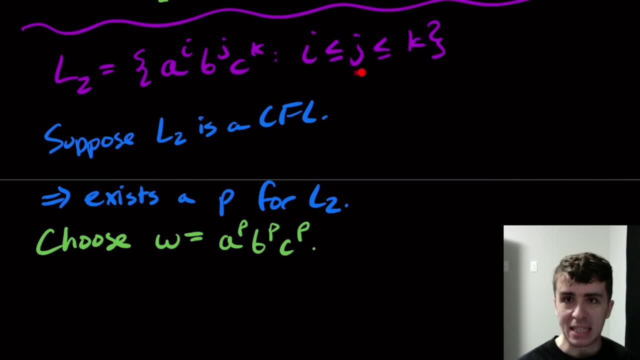 The key is that we want to break these conditions, So my advice here is to pick strings that are right on the edge of not being in the language anymore: If I, If I have 1, 1,, 1,, 1,. 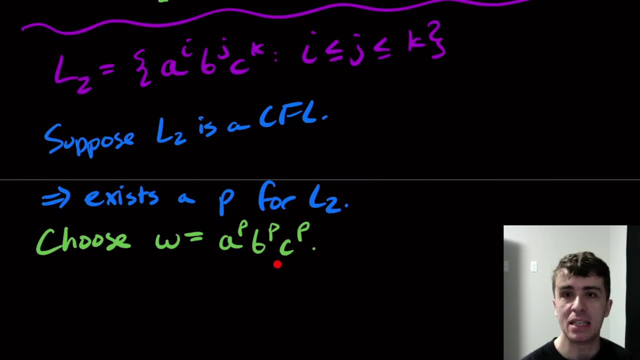 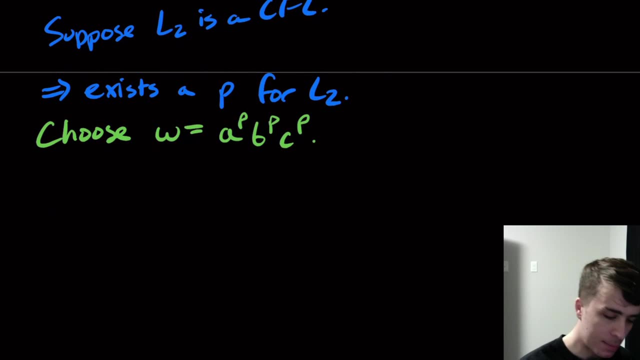 one fewer b or one fewer c than this, then I get out of the language entirely, which is exactly how we'll actually prove this, by the way. Okay, so how are we going to prove this? So we're going to again look at all decompositions. I'm going to shorthand it again: u v, x, y, z. 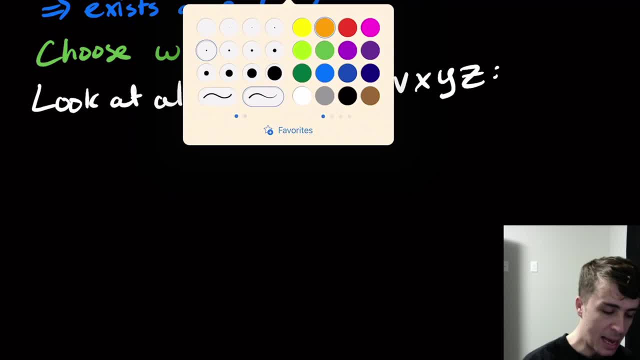 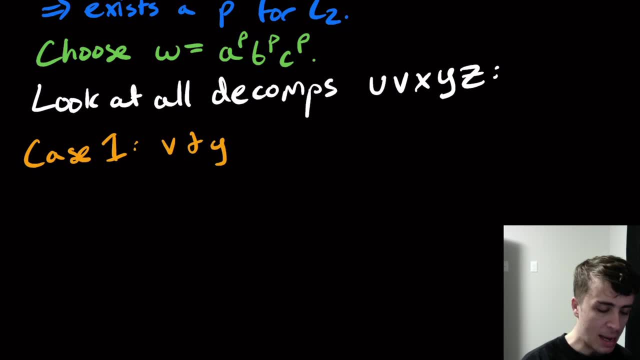 So we got to look at all decompositions. We got to break them up into cases. So let's assume that v and y are only in the a's right here, So the v and y are only in this first section. Then if I pump up we're putting more a's into the string, which means that we're going to break. 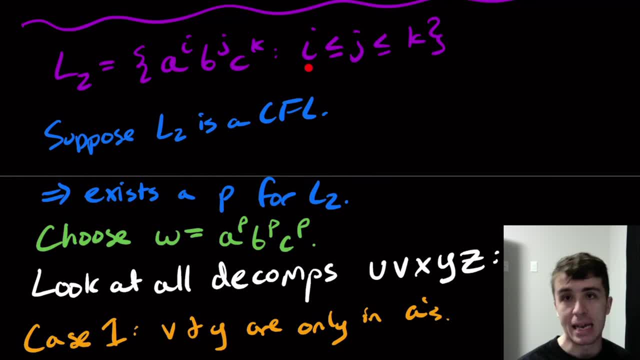 this condition right here. So we're going to have more a's into the string and we're going to have more a's into the string. So we're going to have more a's into the string. So we're going to have more a's. so that means i gets bigger than j, because i and j started out exactly the same. 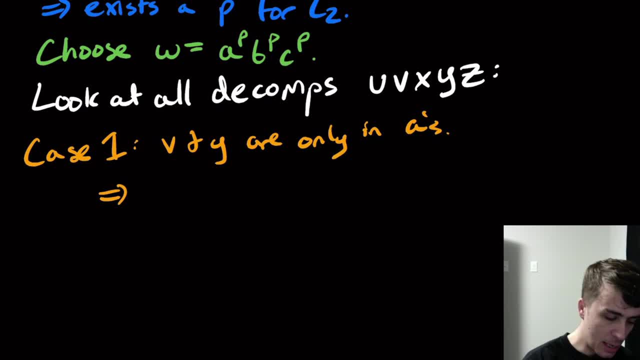 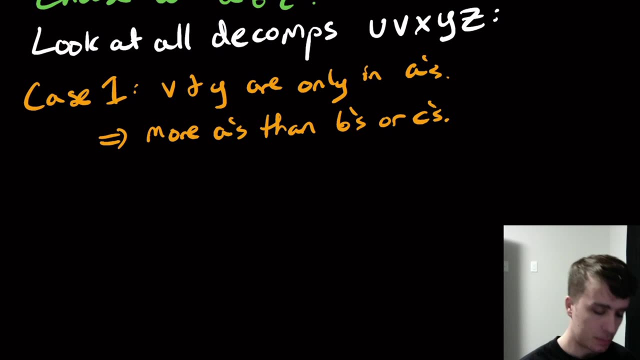 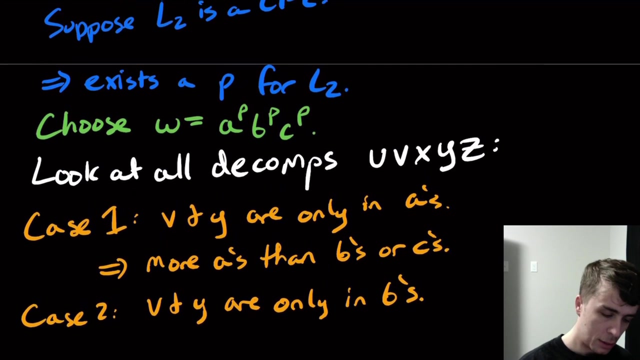 number. So this tells us that there are more a's than b's or c's. okay, which will, which immediately shows that you leave the language. Yeah, yeah, that immediately leaves the language. Case two, v and y are only in the b part. So if it's in the b part, then what we can actually do. 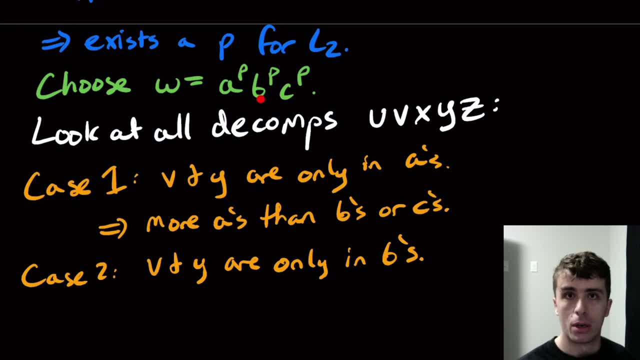 is, you can actually pump either direction, either up or down. Why? Because if I pump up, that'll put more b's into the string, which means we'll have more b's than c's, because they're only in the b part. If I pump down, take the string and I pump up, that'll put more b's into the string. 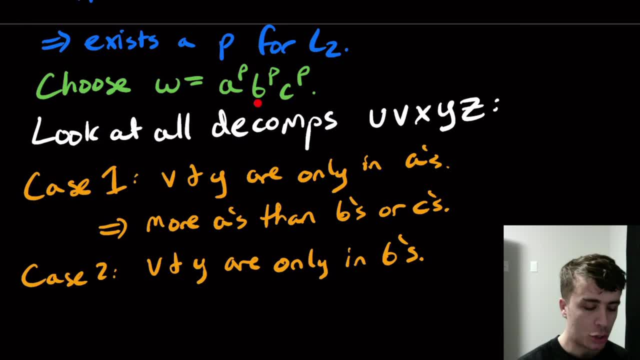 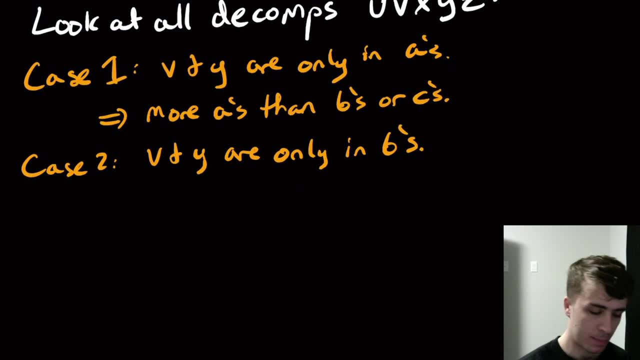 some b's out of the string, then I'm going to have more a's than b's, even though I didn't touch the a's because they had the same number to start with. So oh, I should have said: if we pump to, i equal to 2. And in fact any other value other than higher than 2 also works. 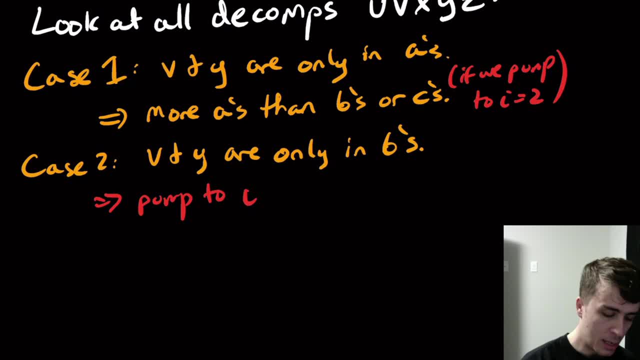 So pump here to i equal to 2,, just as an example. Then here, what will happen is that we'll get more b's than c's, which will, which breaks the condition of being in the language. What about the case of where? 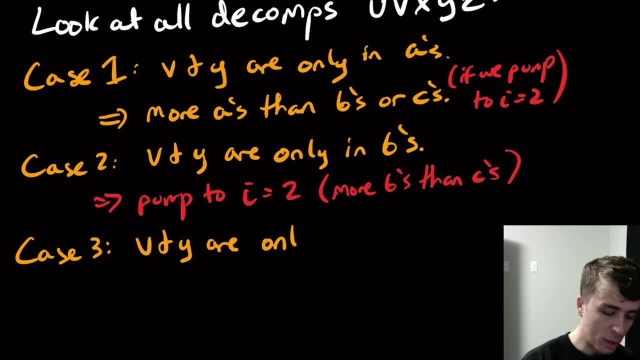 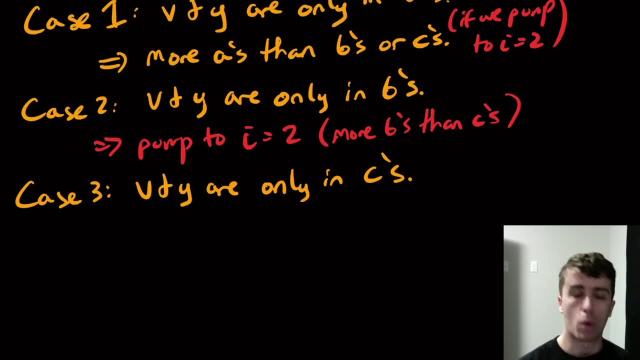 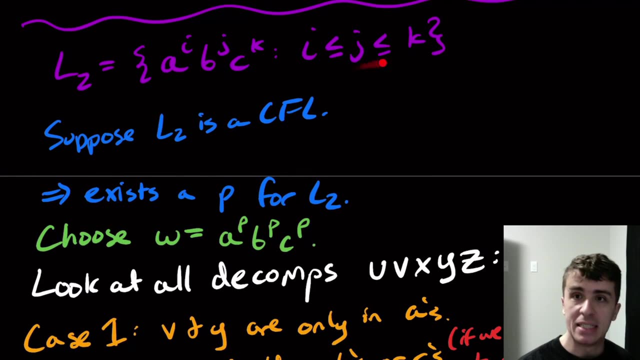 v and y are only in the c's. So this argument of pumping up is i won't work. Why? Because if I put more c's into the string then that will just only make this condition more and more true. It'll just make k bigger. but that's okay, because as long 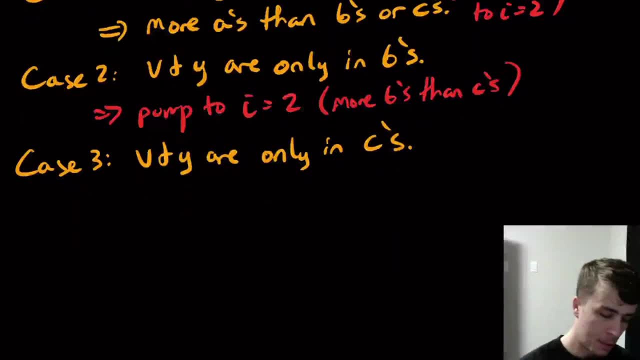 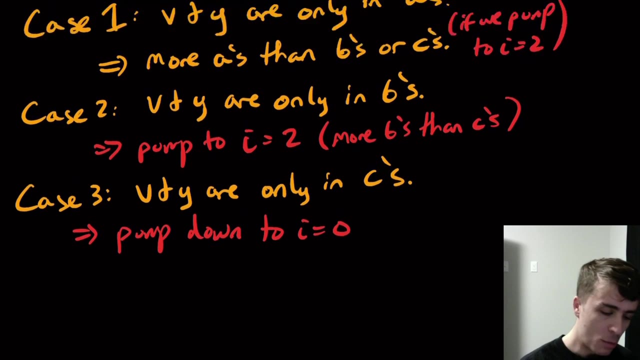 as it's bigger than or equal to j. So what we'll do instead is we'll pump down- Oops, Pump down to i equal to 0.. You can only pump down to i equal to 0. And what will happen is because we have exactly the same number. 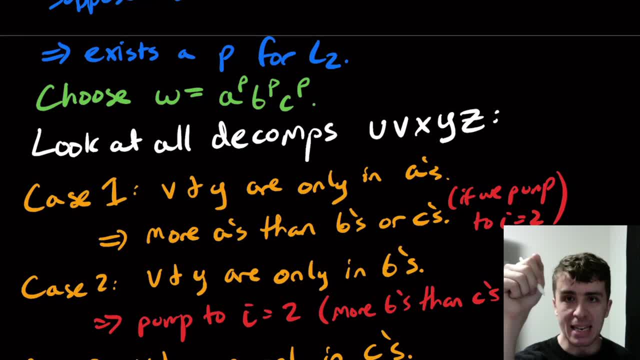 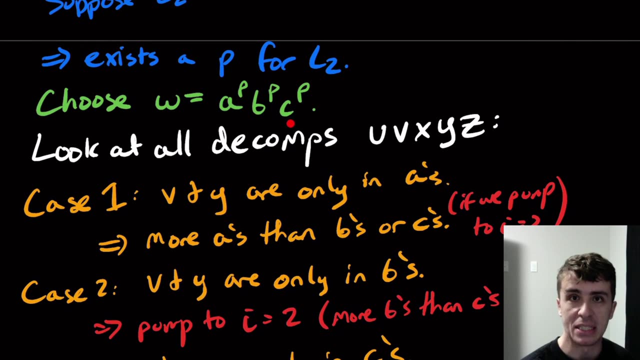 at least one c will be deleted, right, Because one of the two pump pieces is not empty. It can't be the case that both of them are empty. So that means at least one of the c's is deleted, which means that we'll have more b's than c's, And so that will leave the language. So again here. 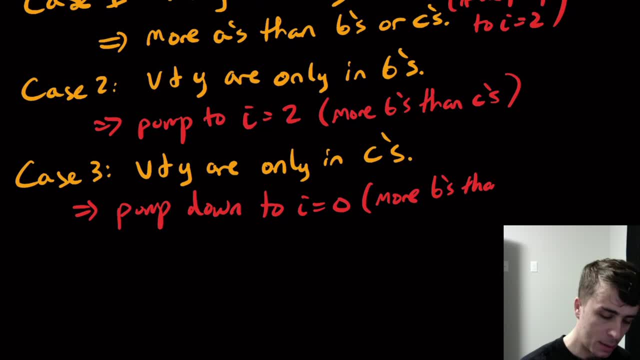 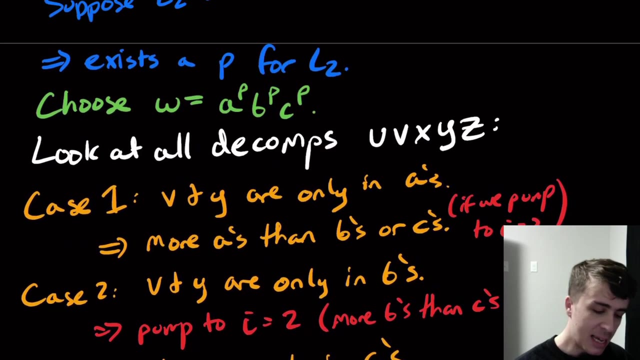 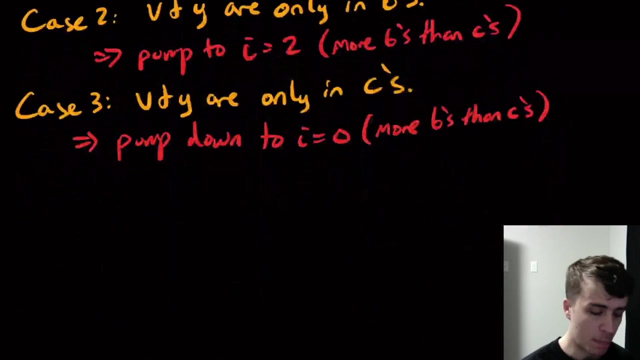 we'll have more b's than c's. It's the same conclusion as the previous thing, but gotten in a different way. Okay, Well, what about the other cases of where it straddles between two segments? It can't have all three segments again because of this gap of p characters, which were all b's. So case four. 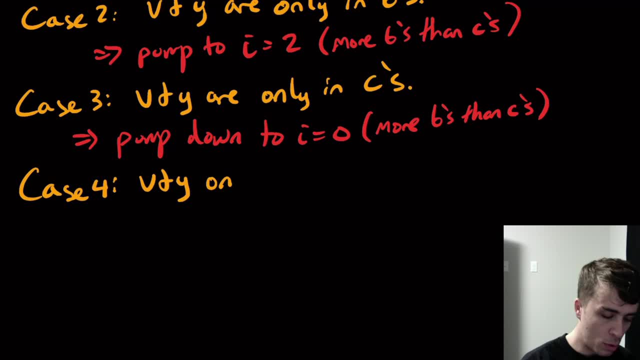 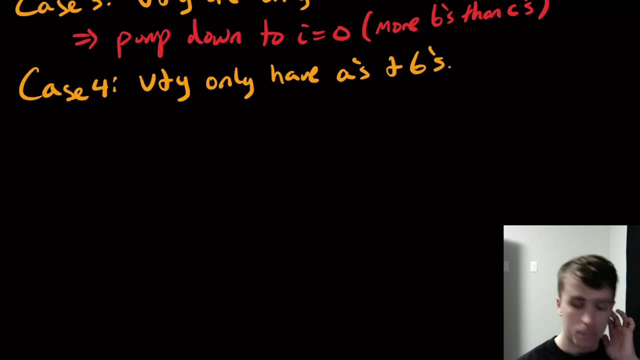 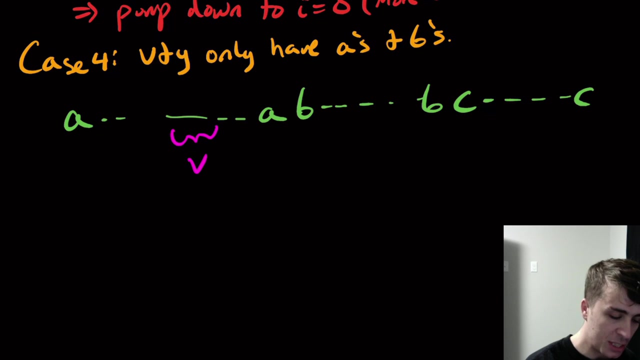 is where v and y only have a's and b's. okay, So let's try to visualize this. So we have a bunch of a's here, b's, c's, And, just like before in the first one we showed, let's just say that the v part's here. 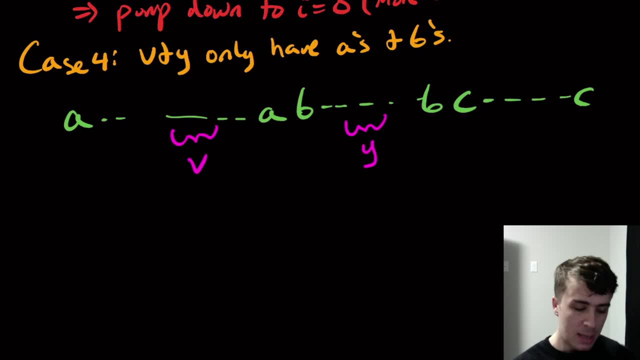 and the y part's here, So it could be that they have the exact same number. So if I pump up or down the v and the y together- remember they have to have the same exponent- then I could have exactly the same number of a's and b's, which actually shows that if you restrict this problem to two, 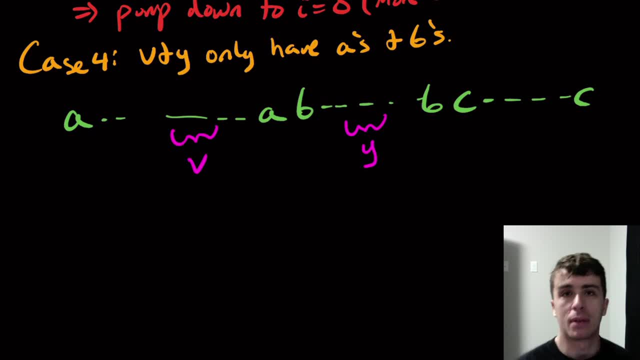 characters instead of three. you can actually keep this to be a context-free language, Or that's actually a way to show that it is, But suppose let's now look at the case where we have three. Well, if I want to break the condition, 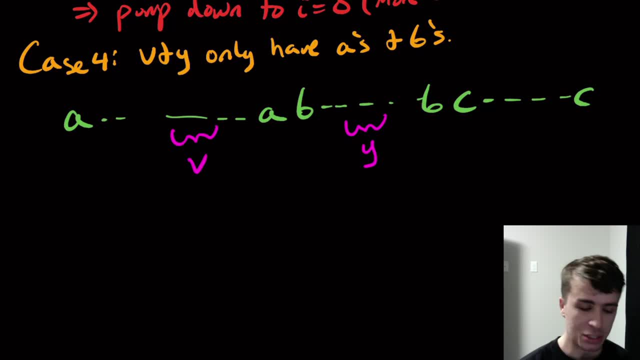 I want to have fewer c's than either b's or a's, So the only way of doing that is to have more b's than c's, because I'm not touching the c's at all. So the key here is to pump, to pump. 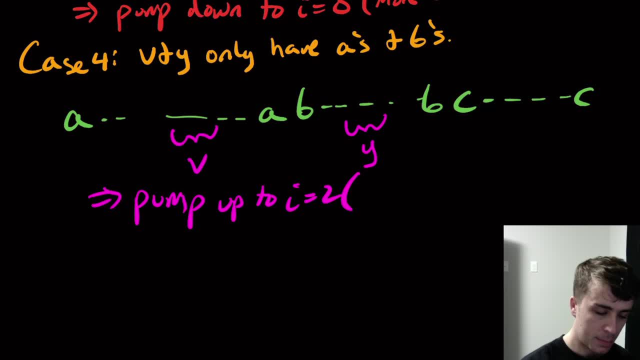 up to i, equal to two or higher, it doesn't matter- Then here we'll have more a's, a's or b's- I don't know which one it is, because I don't know whether I am having a's or b's here. 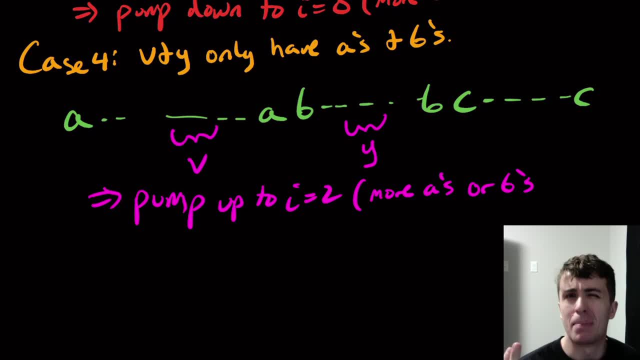 because I don't know which one of these two is non-empty. I could break it up into some sub-cases, but it's enough to handle it here, because I need one of the two segments to have more than the number of c's which I know it will be in this case. So whichever one it is, it will break the condition that the c's and b's are equal. 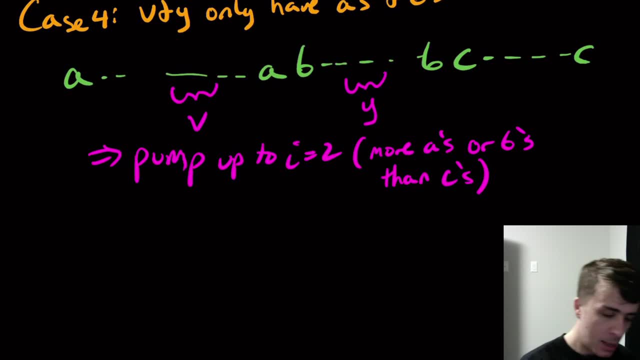 And then finally, finally, in case five, we'll have v and y, only have b's and c's. So now we got to treat this one a little different, because if the v part's in here and the y part's over here, then what we need to break the condition in a different way. 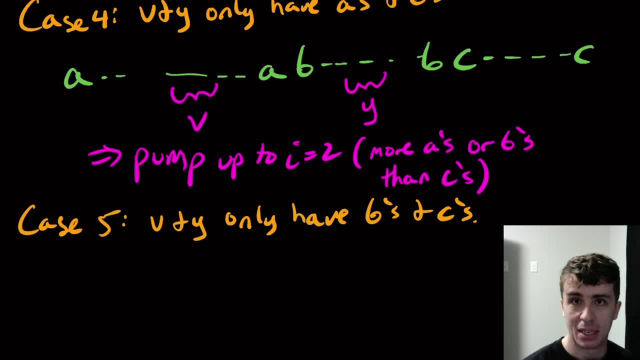 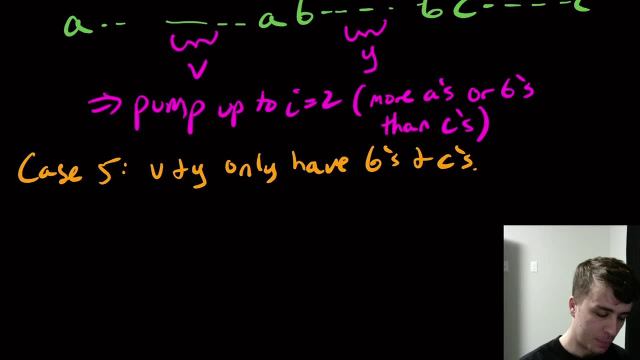 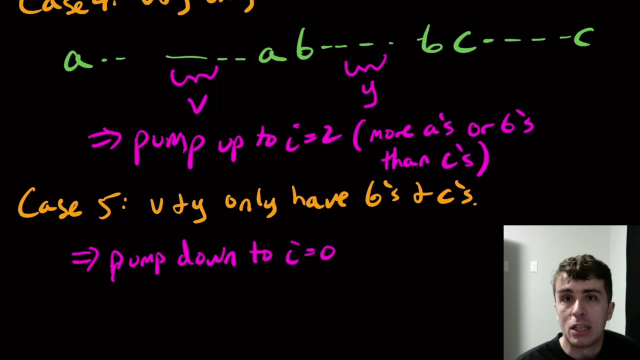 We want to have fewer b's or c's than a's- because I'm not touching the a's in in this case. So we need to do the exact opposite thing. We need to pump down to i equal to zero. So whichever one of these v or y is non-empty. I have no idea which. 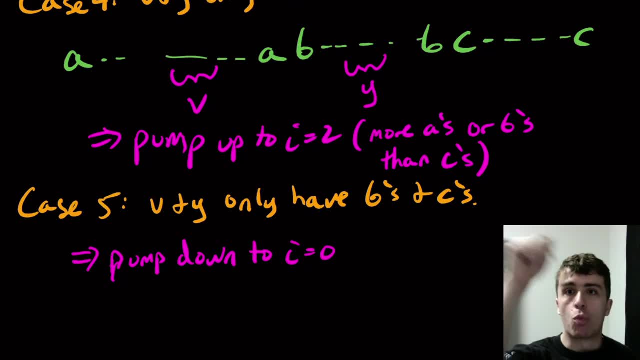 one of the two is going to. when we pump down, will take one b or c with it, or maybe both. In either case, we're going to have more a's than b's or c's, whichever one is the case. 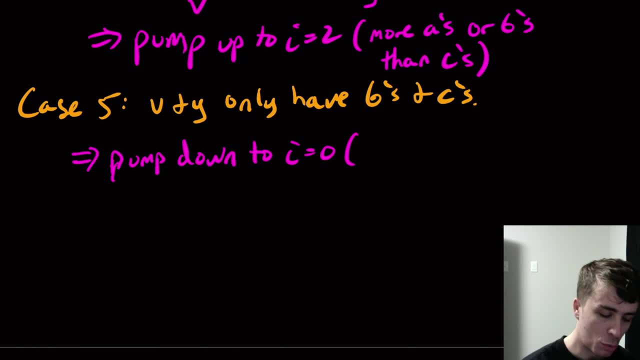 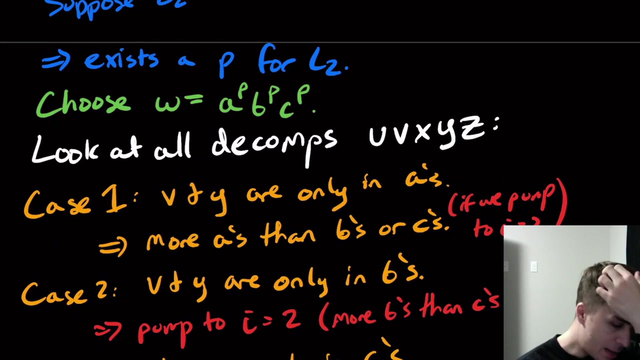 and that'll break the condition to be in the language. So we'll have fewer b's or c's- I have no idea which- than a's. And those are all the possibilities because again I can't have the v and the y part hitting the a's, b's and c's at the same time. 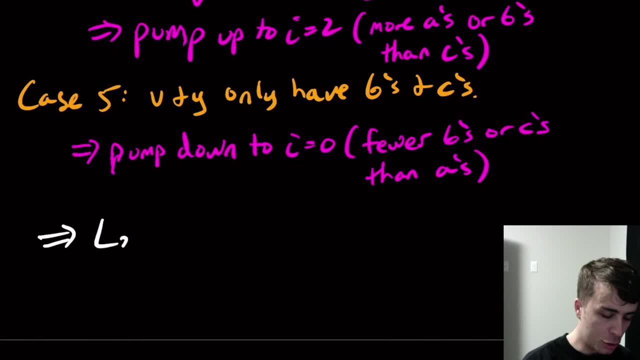 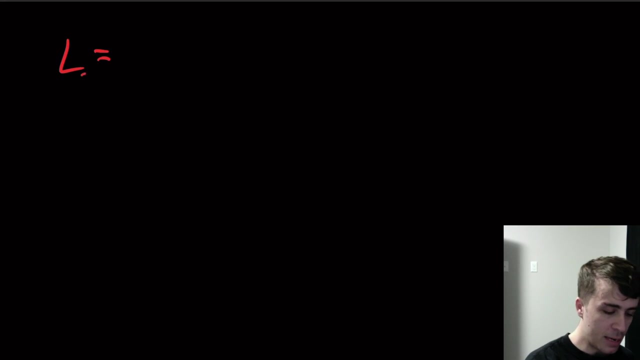 And so that tells us that l2 is not a CFL. Okay, All right, Let's do the third one. So the third one is: very commonly, there's a lot of misconceptions about it. So this is the language ww. so the exact same string twice where w's ain't a. 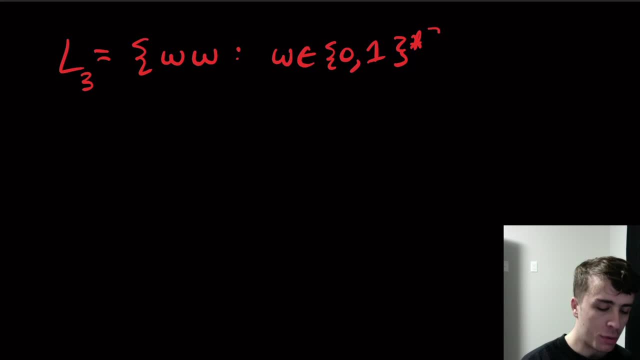 or a, and then so W's are actually behavior-based, or a's, c's are actually behavior-based, and then there's a correct answer, And this is basically kind of a binary string, because this language is a linear counterpart to any possible binary string. Note that, if it was, 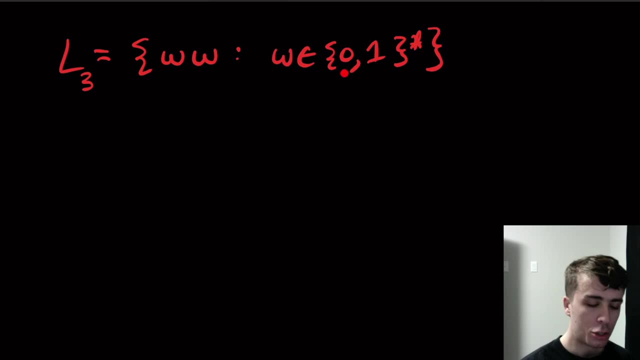 just zeros and not zero ones, then this language would be regular and so therefore it's context free, because it would be all the even length strings. So whatever string we pick here has to have both zeros and ones, because if I just have zeros, then at every point I'm just going to have. 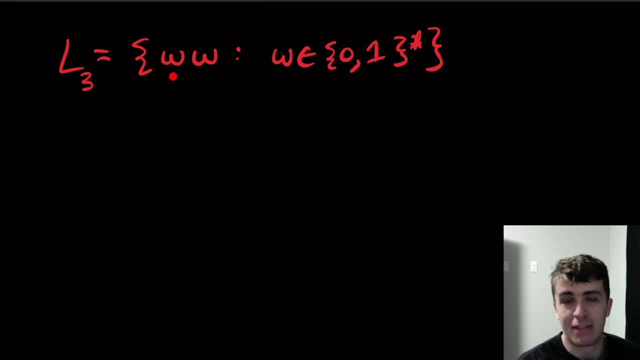 All, even this language only has even length strings. In fact it has all even length strings that have the same two halves. And if you have only zeros or only ones and it's even length, the two halves must be the same. 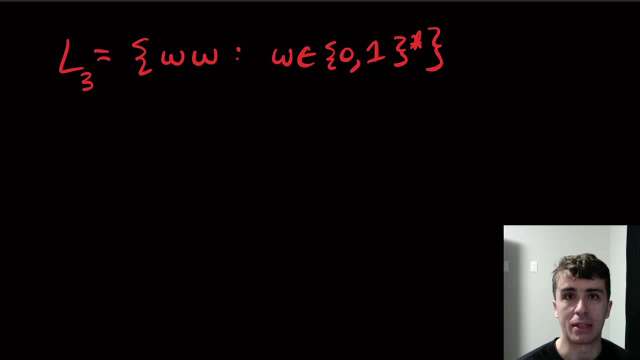 So I must have zeros and ones in whatever string that I pick here. So let's do an example. Let's do this. So let's suppose that L3 is a CFL, Then we know that there exists a pumping constant P for L3.. 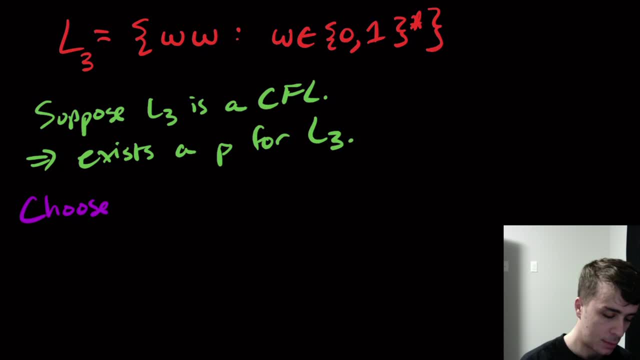 So then now we've got to pick a string. Let's choose zero to the P, So it has to have at least P characters, And I must have zeros and ones in order for this to even possibly work, And I also must have the two halves being exactly the same string. 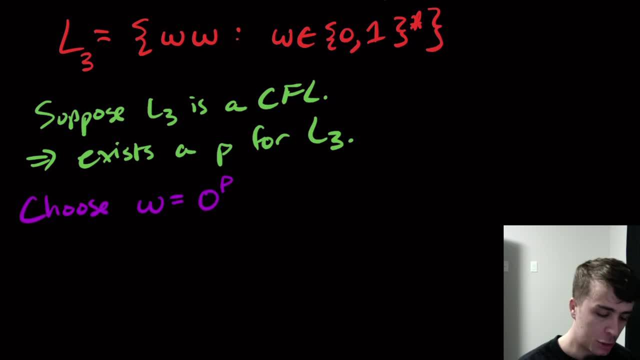 Because that's what this condition is telling me. So if I pick this string- zero to the P1, and I must have the two halves being the same, So zero to the P to the one- It turns out that we can actually find a decomposition that will always stay in the language. 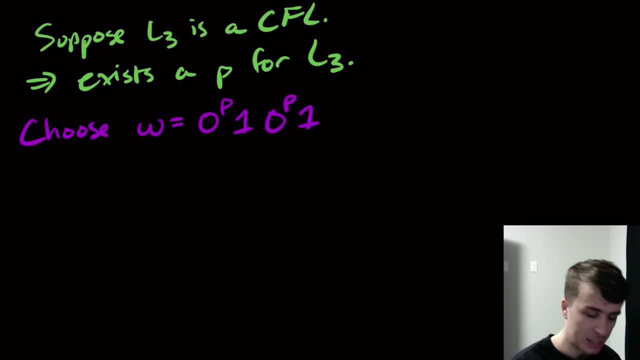 Which is really weird. So here's what the decomposition looks like. So if I have a bunch of zeros, a single one, then a bunch of zeros and a single one, Okay, After that, Then what I can actually do is this decomposition. 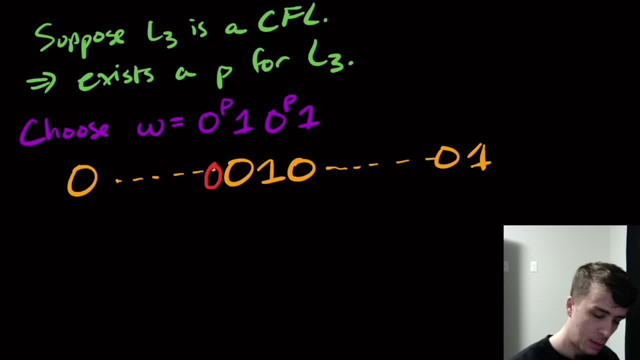 So I'm going to put one zero here, And what I'm going to have is that the U part is right here. The V is a single character, the zero. The X part is the one right here. The Y is just the single zero. 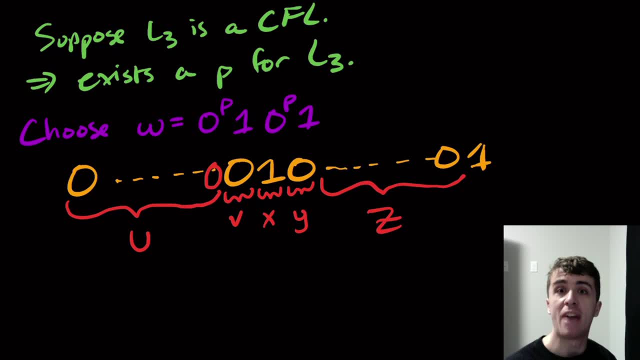 And the rest of it is the Z part. And that's a valid decomposition, Because as long as p is at least three, then we can always pump this string. Why? Because if I'm putting an additional copy or deleting a copy of v and y at the same time, then I'm putting a zero. 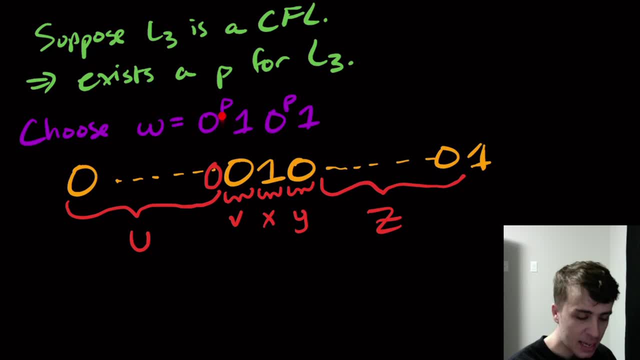 on both ends, or yeah, I'm going to put a zero in this set and a zero in this set, and the two halves will be exactly the same length and they will have the same number of zeros on both sides, and so therefore they are exactly the same. So unfortunately, I can't pick this string, but the idea is very. 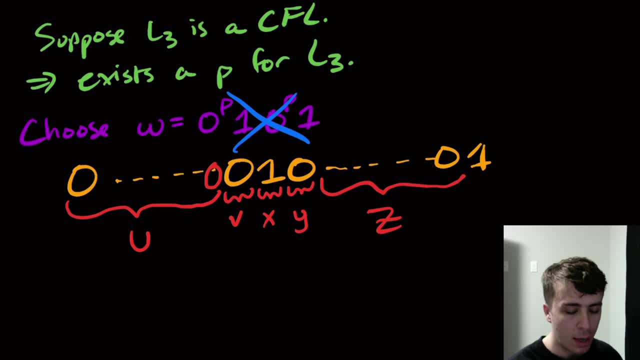 good. The reason why this went wrong is that the v part was in one set of zeros and the y was in the other set of zeros. So if we can make the gap between the sets of zeros big enough- length p- then we can actually force it to only touch one set of zeros at a time or one set of ones at a. 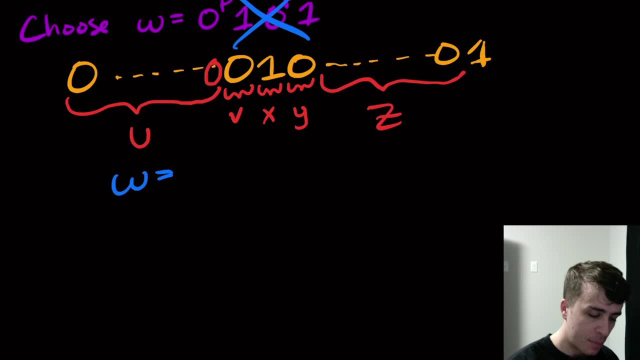 time. So what we'll pick instead is zero to the p, one to the p, zero to the p, one to the p, And this is, of course, of length at least p, and is exactly the same string on both halves, So this is the same. 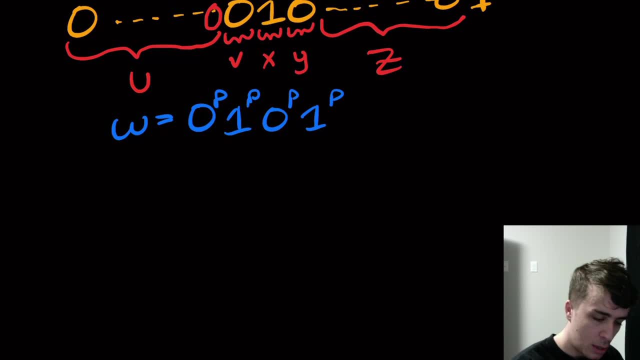 as this, which is pretty nice. So I'm going to put this string on both halves and then I'm going to put the length p in here, and I'm going to put this in here, and I'm going to put this one on the other. 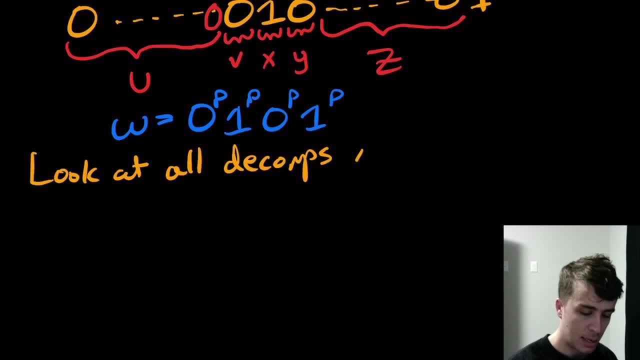 side, and this is going to be just the same as the one that I put on both halves. So what we need to do now is we need to look at all the compositions. so look at all the compositions into u, b, x, y, z again. So let's see. we can actually handle this into two cases: believe it or not, reduce it. to two cases. You could handle every single possible case, but this is a lot easier. So when you look at the, So with the dy昀 you're going to have the two side of the Pygmalion and you can't just pick the first set of zeros by one. 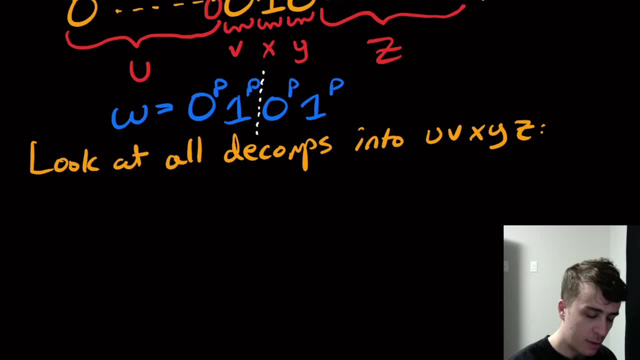 I'm going to do is I'm going to look at this string in two halves. I'm going to call this the left half or the first half, and this is the right or the second half. So case one is that v and y- actually I'm going to break it into three cases- are only in the first half. 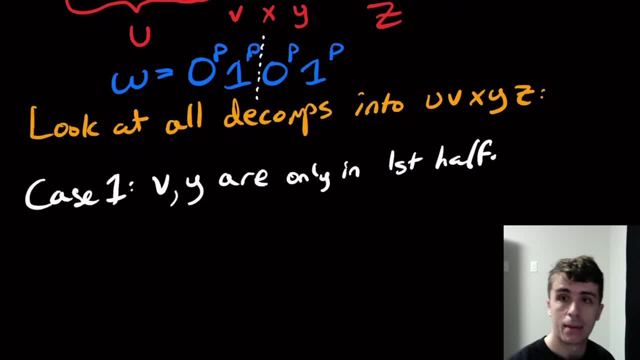 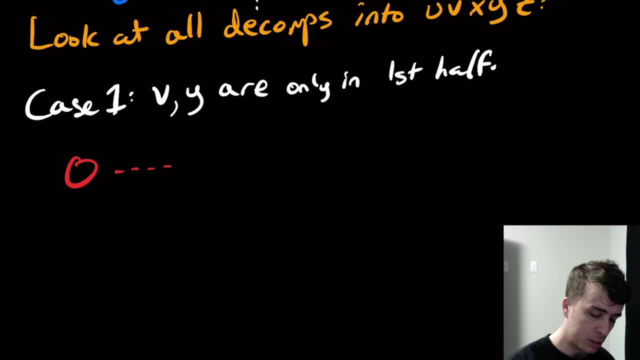 Okay, they're only over here, so let's try to visualize what this looks like. So we have a bunch of zeros at the beginning, then a bunch of ones, then a bunch of zeros, which is starting the second half, and then the set of ones at the end. So again, here is the midpoint of the string. 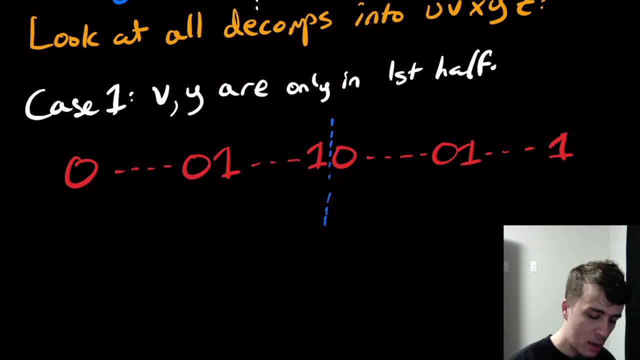 and so v and y are over here somewhere. So let's say v is here, y is here. I don't really. this case is telling me that it doesn't really matter where v and y are. As long as they're over entirely on one side, then that's. 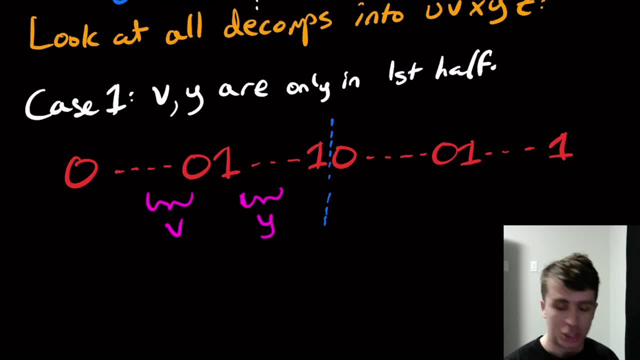 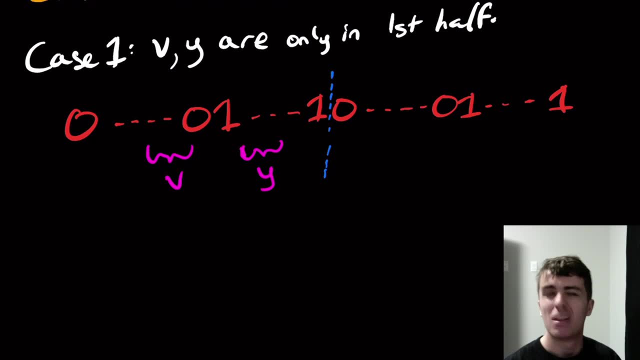 okay, So let's see what happens. So it turns out that you can pump in either direction here. But let's visualize if we pumped up. Pumping down works very analogously, So let's visualize what happens. So what happens if we pump up to i equal to 2? Then what happens is we're putting 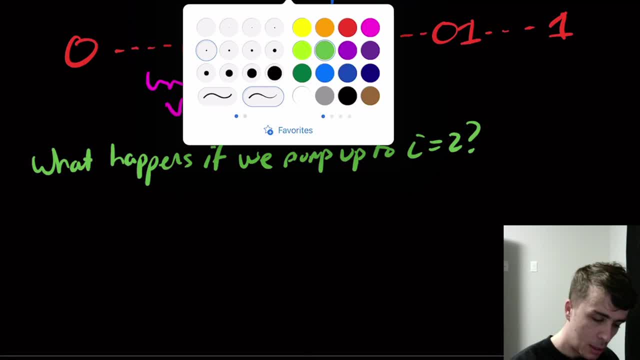 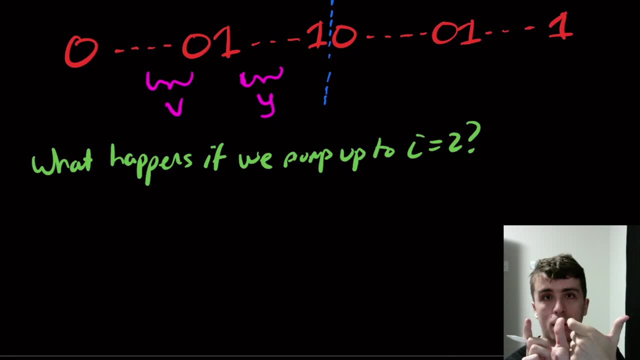 more of v and y into the string. So that tells us that we, in order to stay in the language, the two halves must be exactly the same right. And I'm not going to worry about whether we're putting in an even number of characters If we put in an odd number. 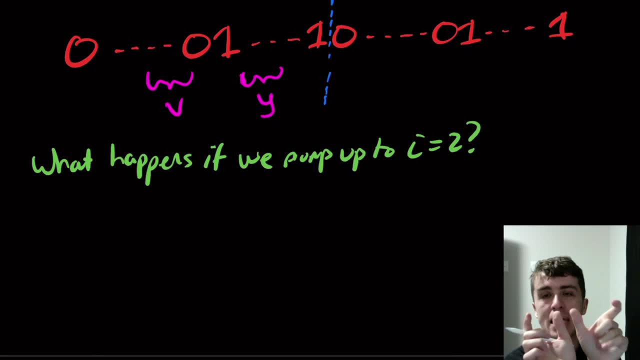 then the whole string's length is odd, And so it can't be have two halves that are exactly the same. But let's just assume, for example, that v and y contribute an even number of strings. But it won't actually matter, So the key is this. So we're going to look at the string again. 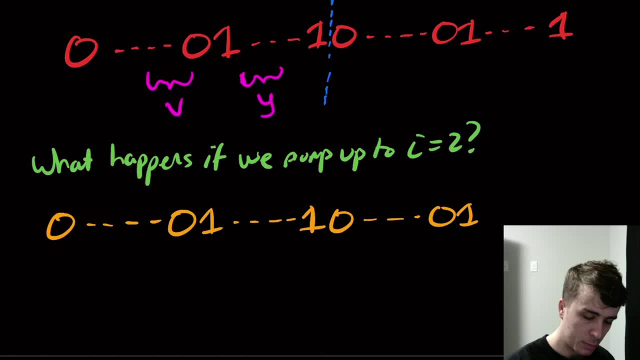 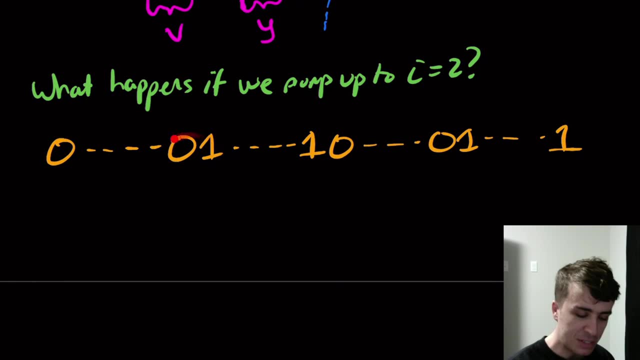 So here's zeros ones, zeros, Ones. So what happened is, well, if we put more of the left stuff here, then, if you think about it, the original midpoint of the string which is right here. so this is the original midpoint. 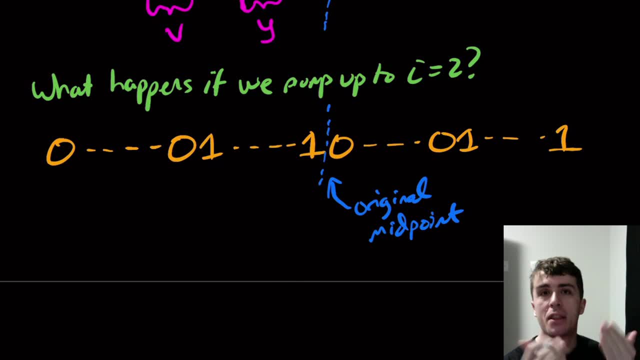 Well, it must have moved somewhere because the string actually got longer or it changed length. Okay, So the string actually got longer or it changed length. So if we put more of the left stuff matters, it changed length so that it must have moved somewhere. if you think about it, there's. 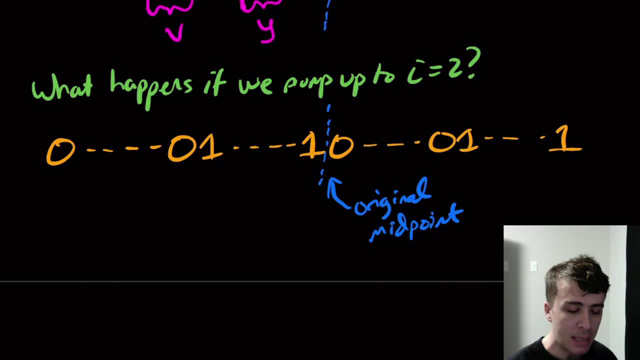 more characters over here. so that means that, then, are over here. so that means that this midpoint actually moved to the left because in order to have the two sides have exactly the same length, so that means that the mid, the new midpoint, is over here somewhere. so this is the new. 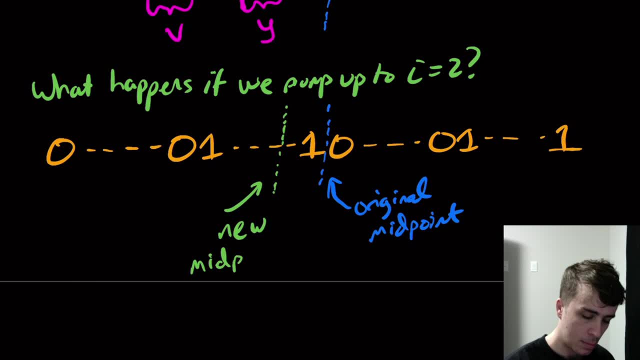 midpoint, and here's the key idea, because it moved. the right side here must start with a one. okay, and you can prove that. uh, you can even prove more than that, but it's: the right side starts with the one, but the left side starts with the zero, which is a contradiction. so the right side 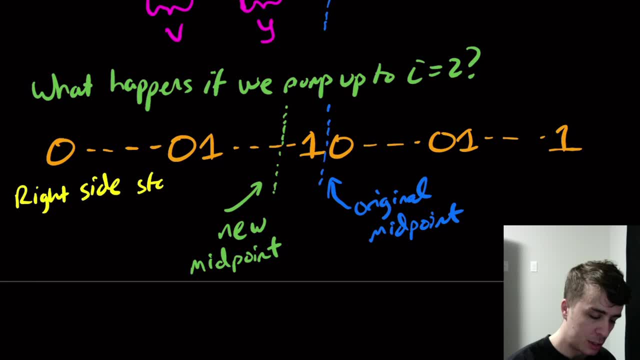 starts with a one and the left side starts with a zero, and the right side starts with a one and left starts with a zero. so that tells us that the two halves cannot possibly be the same, because they start differently. and you can actually prove more than that, but that's enough to show that the 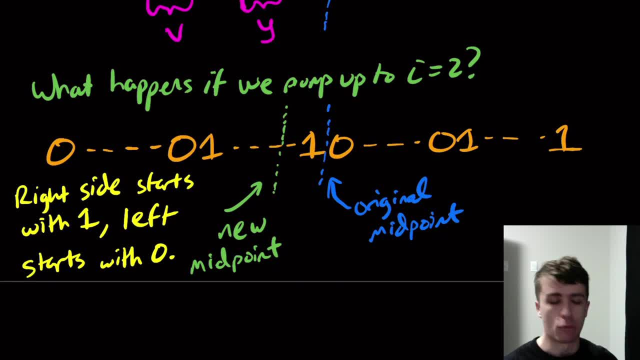 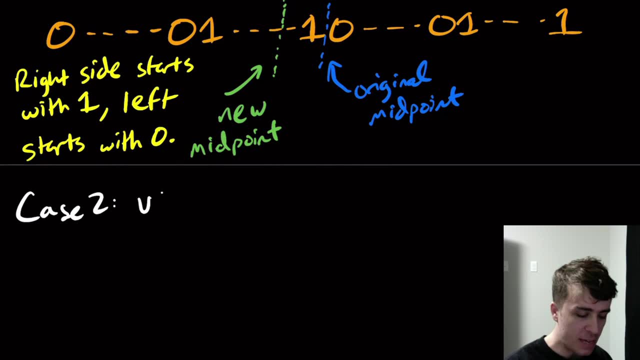 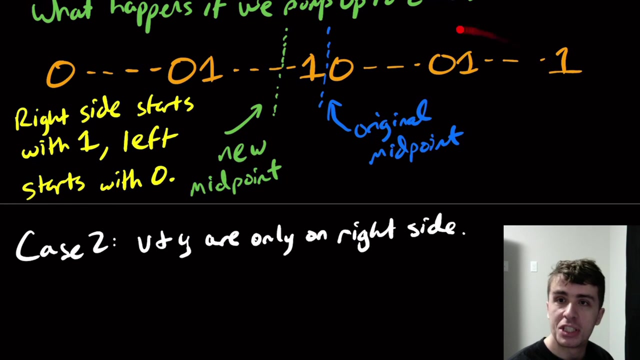 resulting string can't possibly be in the language. and actually the same logic works if we look at case two, where v and y um are only on the right side, because if we pump up to i, equal to two. now in this case there are more stuff on this side if 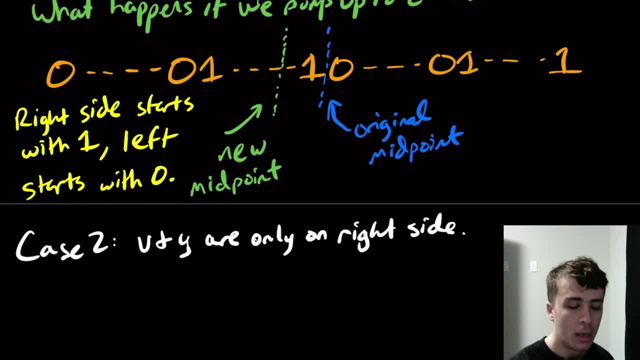 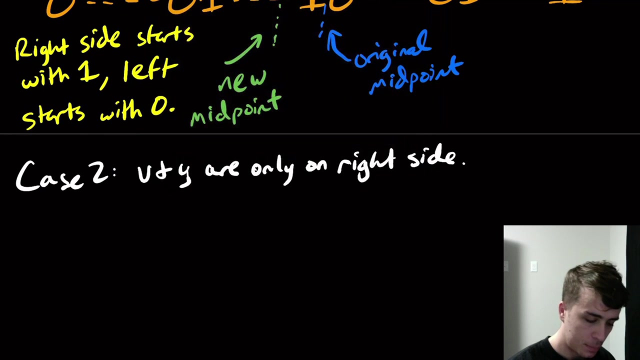 we put more onto the right side, because that's where they are here. the original midpoint was here, but now the midpoint has to move. this way. that means that the the left side ends with a zero and the right side ends with a one. i'm getting notifications, so, uh, let me write what happens here. so pump up to i equal to two. then what happens is: 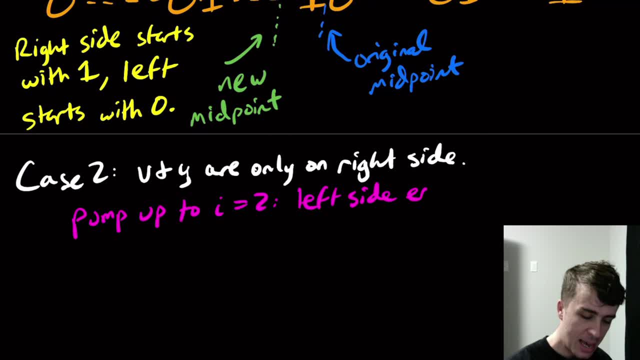 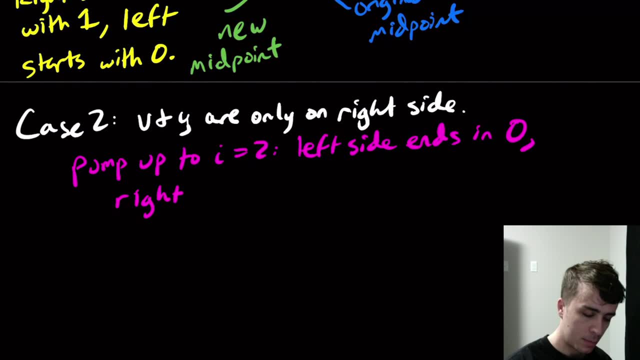 the left side ends in a zero because the midpoint moved, and the right side ends in a one, and so the two halves cannot possibly be equal to each other because they end differently. it's a very similar conclusion, but it's not the same conclusion. obviously the first. 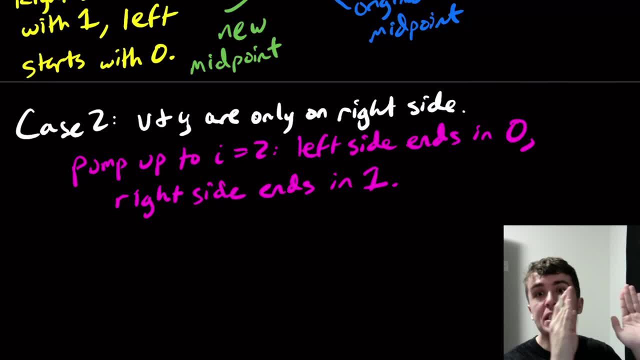 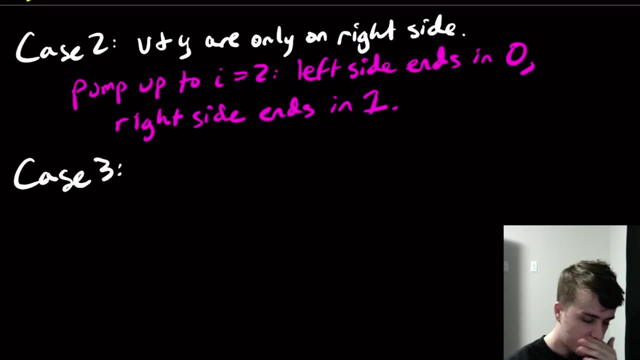 one is the they started differently, now in this case, they end differently. but now there's one other case, which is that uh, v and y are not the same conclusion. obviously the first one is that the left side ends with a zero, so that means the right side ends with three zero one, so that means 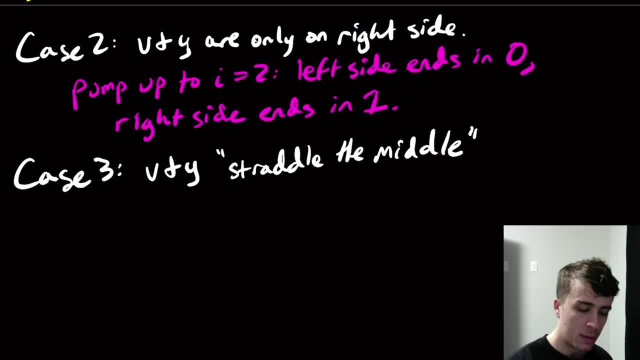 that the bottom part ends with a one and the others end with zero. so that means there are single ائ. can you can you see if you do it correctly in this case? you can you see that the bottomاد27 doesn't end in a one and the canned sharing, so that area ends in a one and the others end. 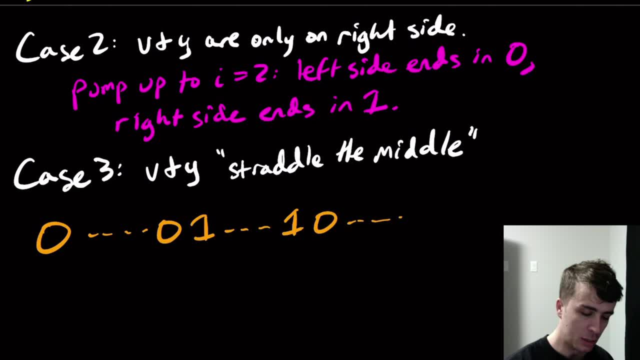 with a zero that mean this is an safe right- Authuty examples up there again. so you're just doing the same thing. so if this case, you put all those points together and all those out there and you're just doing the same thing over and over and over again. that's how you want your м data to be. 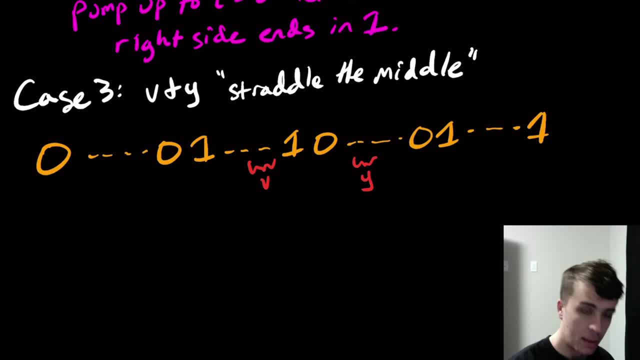 v part is here and the y part is in fact here. So what are we gonna actually do here? Well, let's see what happens. Let's try to pump up again. It'll actually work. So let's pump up to. i equal to 2.. 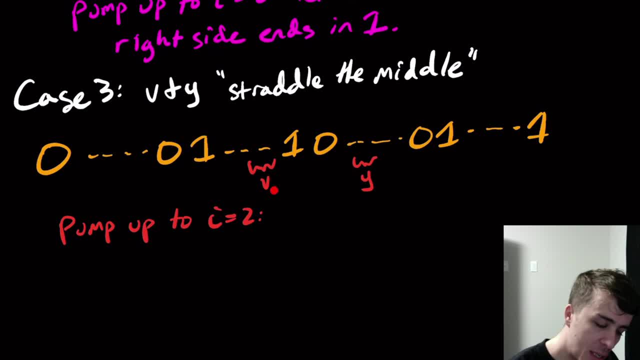 Then what happens is that you can actually show that if we're not in the first two cases, then both v and y are both non-empty in this case- Although it won't actually matter, But we can show that they are are non-empty, So let's just think they're non-empty. So v is non-empty, Y is: 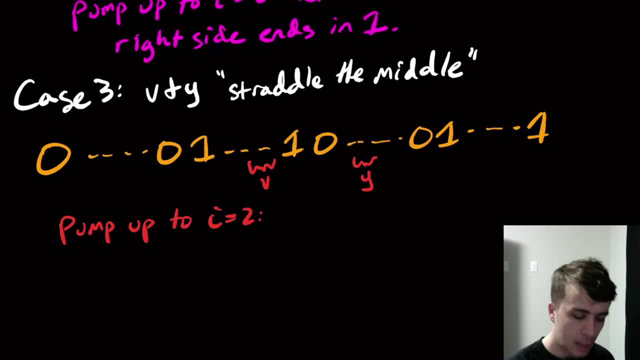 non-empty. If we pump up to i equal to 2, then that means we're putting more ones here and more zeros here. So here's the key idea: If we put more ones here, then that means that this second case is going to be equal to this set of ones. This set of ones has to be identical to this set of ones. 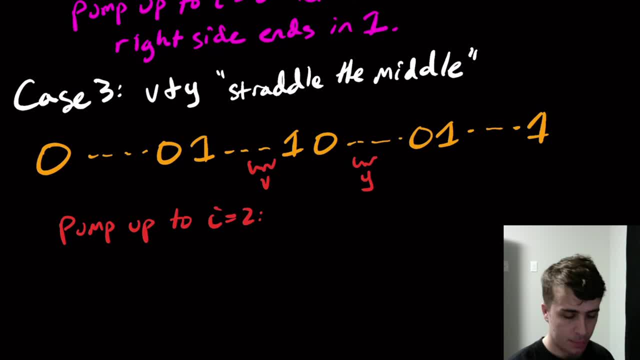 because they can't both be on the same side, unilaterally on the same side, And for that reason, this set of ones cannot possibly be equal to this set of ones, because this originally had the same number as this and we're putting more ones into the string. Similarly, if we're putting 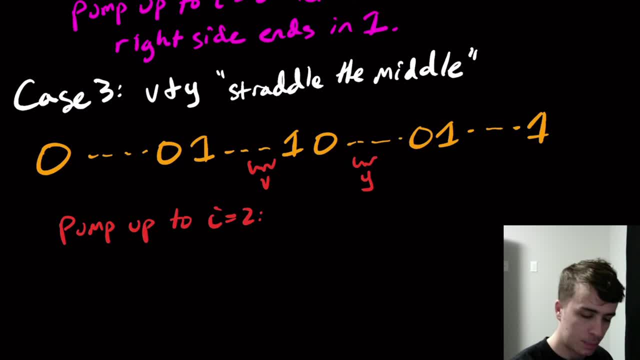 more zeros here, then it can't be equal to this set of zeros which we didn't touch. So here, just as an example, the number of ones on the left side is not equal to the number of ones on the right side, And similarly for zeros. Okay, and so that shows. 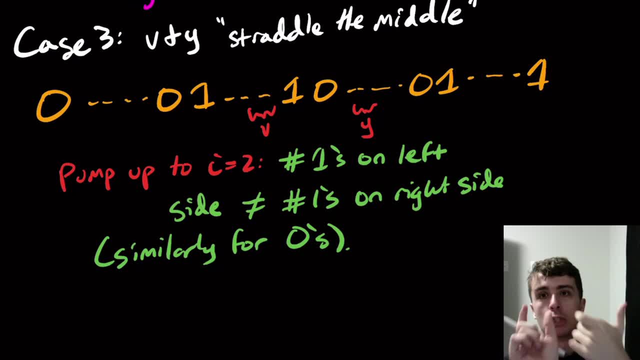 that this string cannot possibly be in the language, because the two halves cannot possibly be the same, because the number of one of the characters is not the same, Never mind whether it actually is in the right order, but they can't possibly be the same. Okay, so in all, 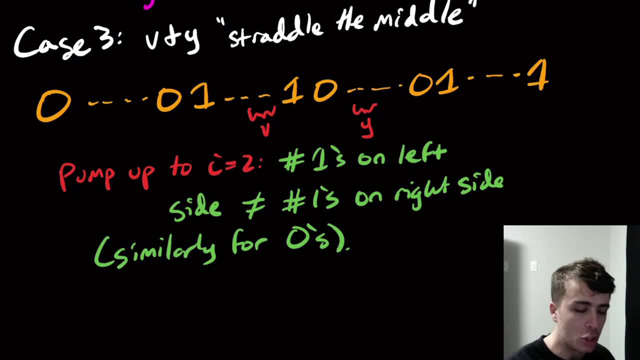 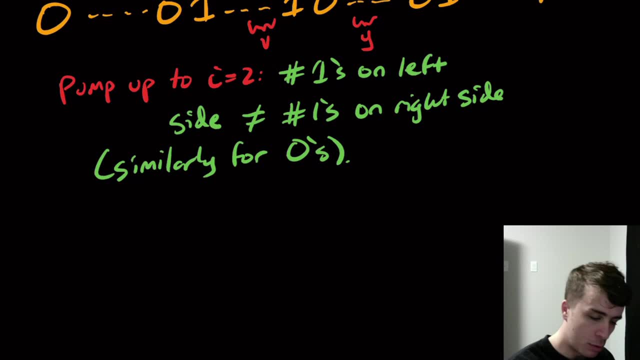 those are all possible cases, because each of these ranges has p characters, so I can't hit three of the sections at the same time, And so in all cases we have shown it to leave the language, And so L3 is not a CFL. All right, so now let's do one. 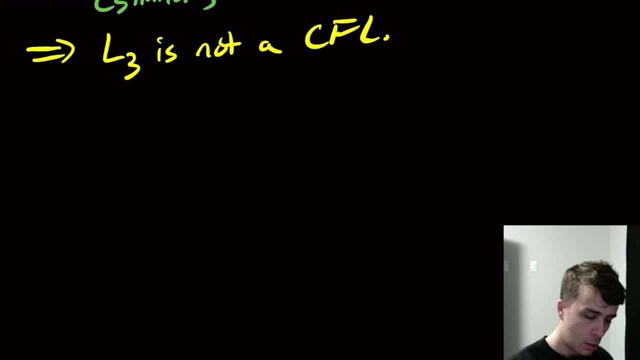 that's actually kind of really interesting. So we're going to hold an election. No current events are motivating this, by the way, just a disclaimer. So we're holding an election here and the string string that we have is in the set: a, b, c, d, whole thing star. so it's just a string of a's, b's, c's. 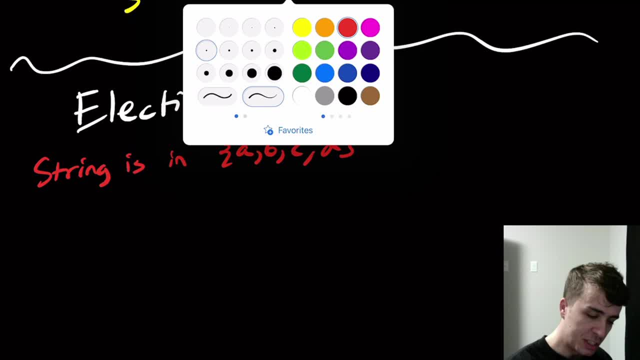 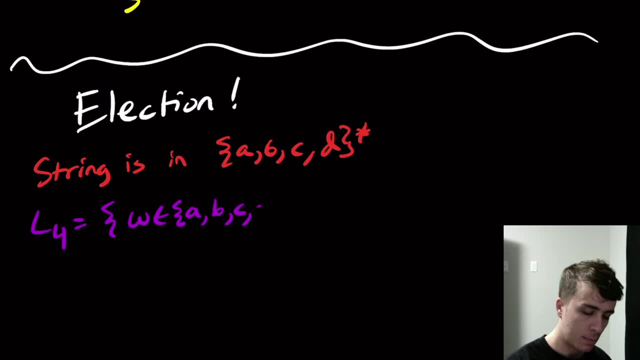 and d's, and the set that we're interested in is the set of all w, all strings w in this set, such that the number of c's- as an example it could have been a's, b's or d's, but it doesn't matter- the number b, the number of c's is um- is more than the number of a's, b's or d's. 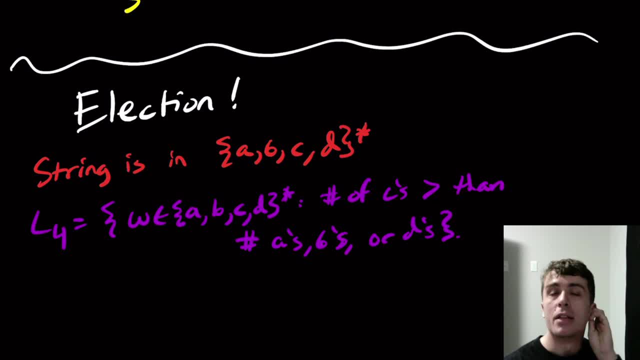 okay, so, uh, the number of c's is more than the number of a's, b's or d's here. okay, the number of c's is more than the number of a's, b's or d's here. okay, so the number of c's is more. 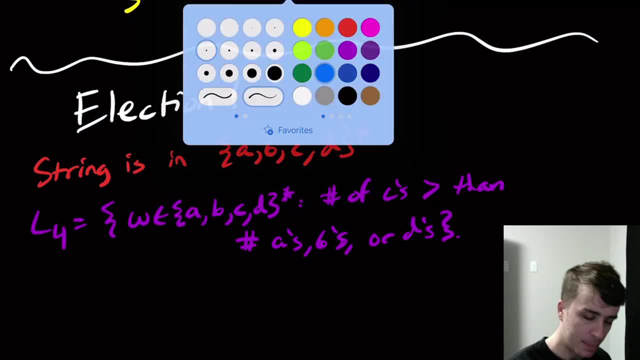 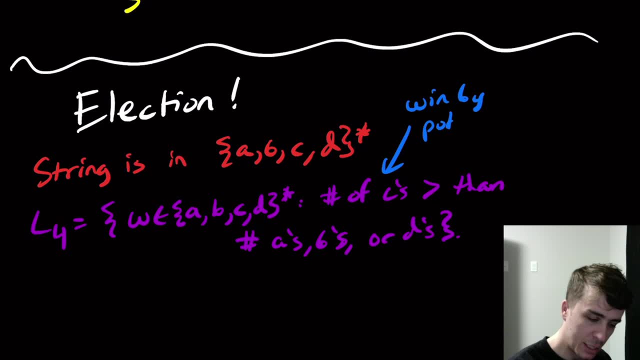 this is what is called, uh, winning by plurality. so a win by a plurality can't spell plurality. plurality, it's not majority, because we're not requiring that the number of c's be at least, uh, fifty percent of the length of a string is what we're just. 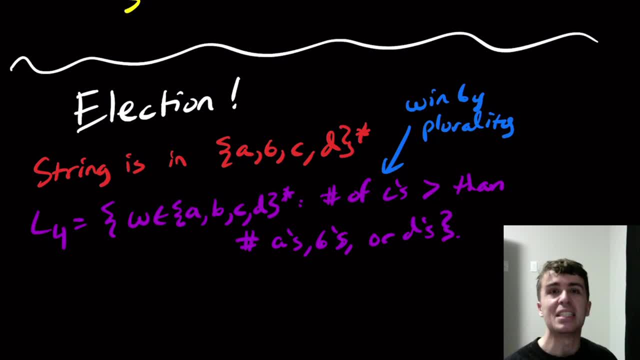 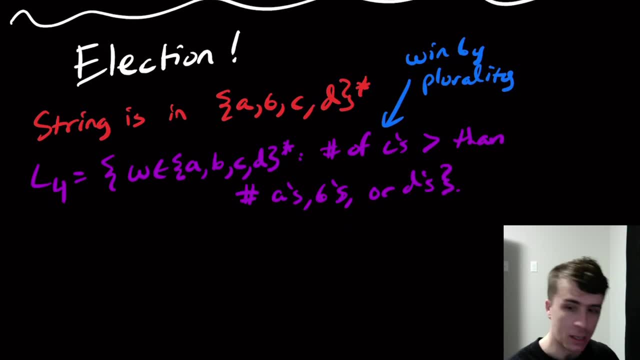 saying is that the number of c's is, at least is- bigger than the number of a's, b's and d's, so c technically got the most votes, and so what this should tell you is that a context-free grammar, or anything like a pda or something, cannot possibly, um, have this language, and so we. 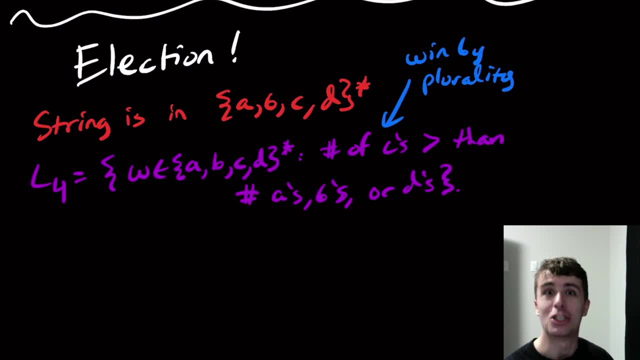 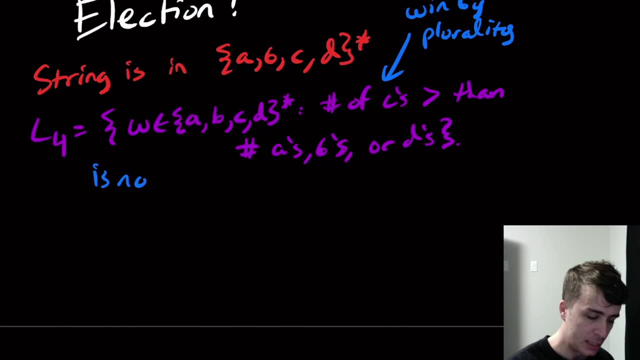 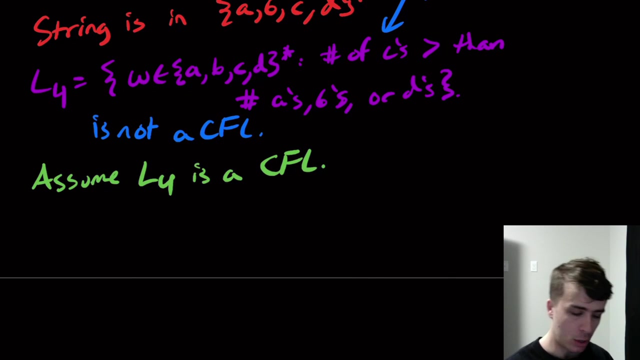 shouldn't use context-free grammars in elections. that's your psa for the day, all right, so what i want to show is that, uh, this thing is not a cfl, so let's uh assume that l4 is a cfl and what we'll do here is we are going to 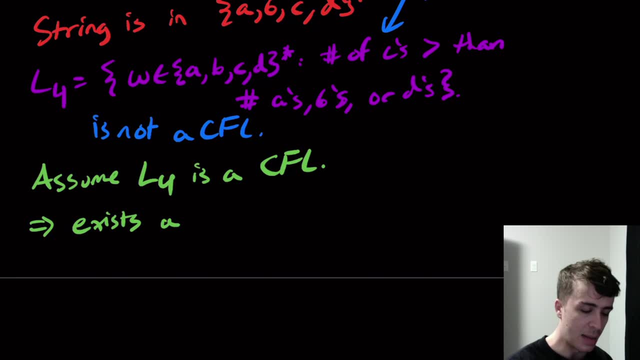 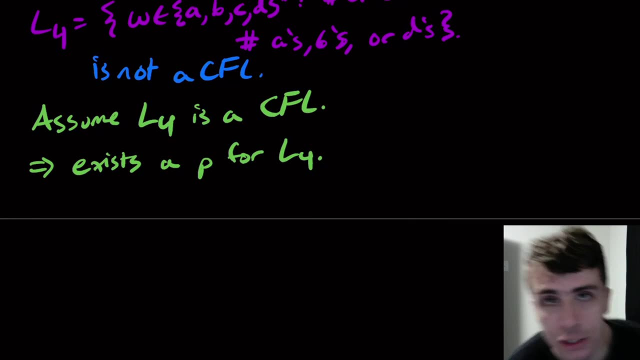 we know that there exists a p, a pumping length p, for l4. so now we need to, uh, pick a string that's in the language and long enough. so remember my advice, which was to pick a string that's just barely in the language, and it's just barely in the language, and it's just barely in the language. 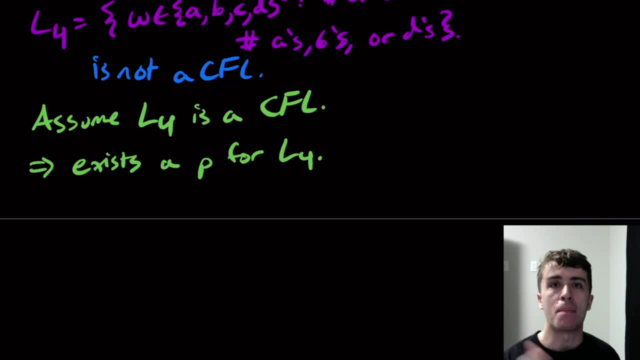 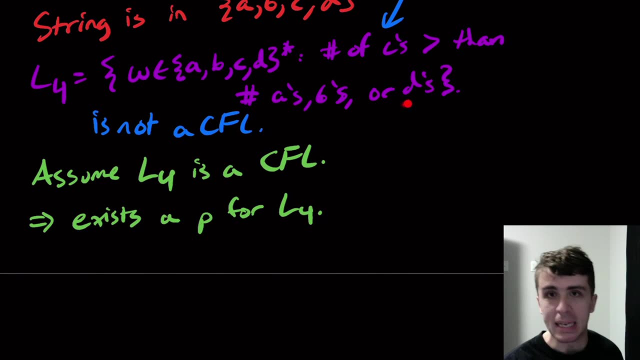 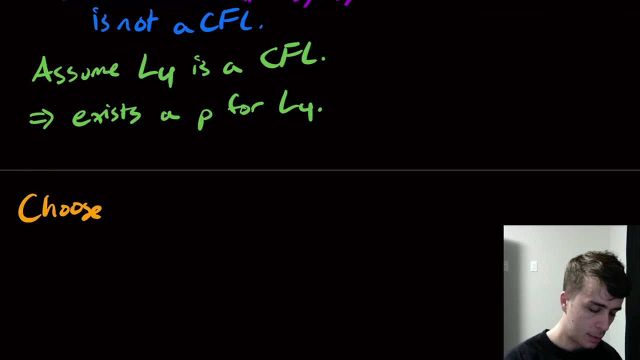 any small tweak is going to have it not be in the language anymore. so if we want the number c's just barely bigger than the number of a's, b's or d's, then what i, what i'm going to do, is i'm going to have the string to be c to the p, plus one a to the p, b to the p, uh d to the p. okay, uh, the a, b and d. 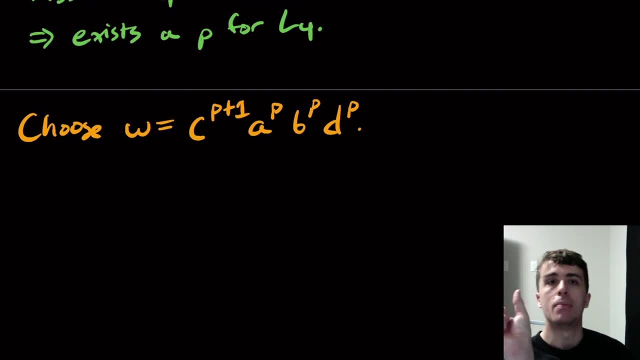 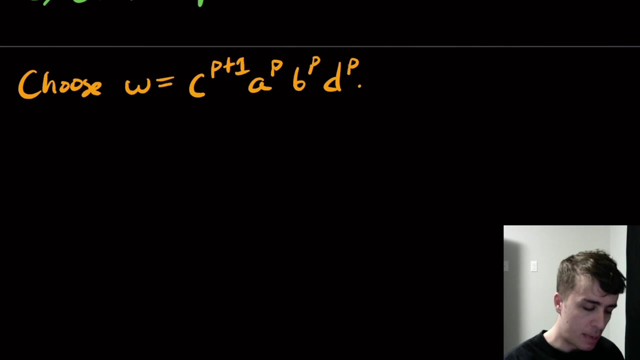 doesn't matter. in fact, the c order doesn't matter either, because, remember, we can technically pump anywhere, but it's just um, i like putting it at the beginning: uh, here, okay, so, uh, what do we actually do here? so we gotta again look at all the possible cases. so look at all decompositions. 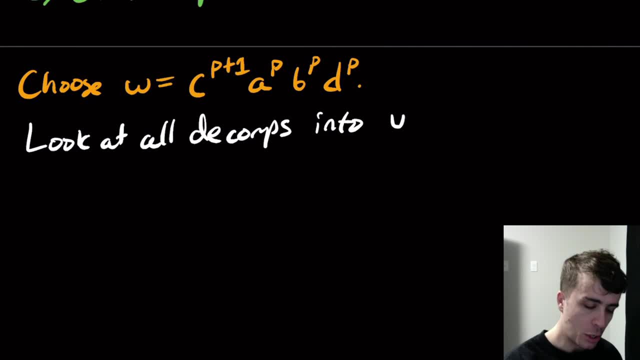 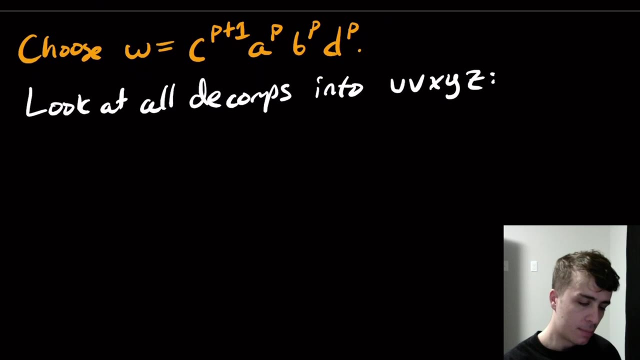 into u, v, x, y and z, and so we want to have it that c doesn't win by plurality anymore. it could be that one of the others wins by plurality, but we want c to not win by plurality, okay, so what will happen? so let's look at some cases. 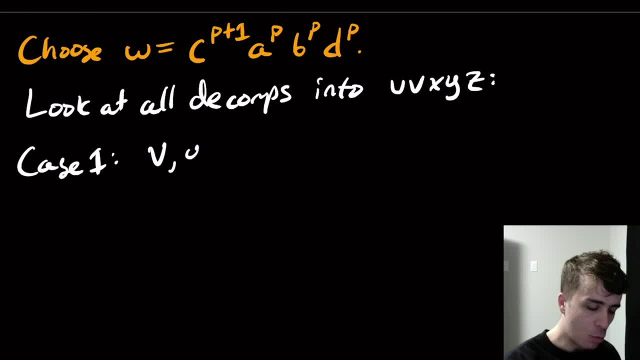 so case one is v and y are only in the c's. so, since it's barely more, if i try to pump more into this, then what i'm going to get is more c's, and that's not going to ever leave the language. i want to leave the language. 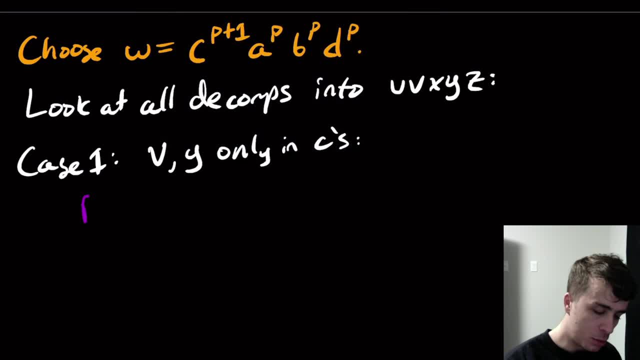 so here, what we need to do is to pump down to i equal to zero. so what will happen there is that, um, yeah, so then what we'll have is: uh, actually i'll write it this way- so the number of c's, because we take at least one away, but it could be one, the number of c's is: 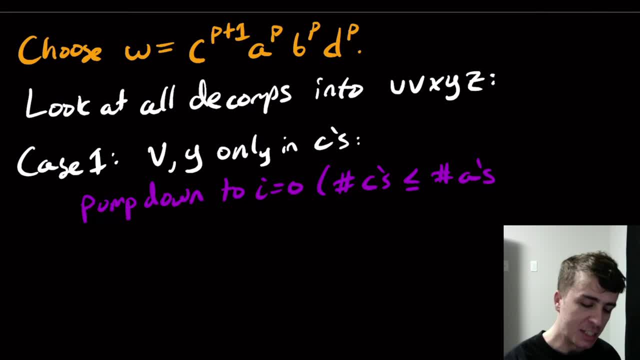 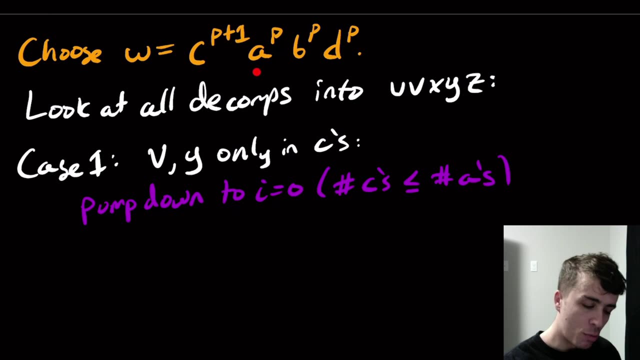 less than or equal to the number of a's in particular, and so, uh, that that clearly shows that c couldn't have gotten more votes than a did because, um, it's less than or equal to it. but if we think about v and y being anywhere else, the a, b and d are all symmetric to each. 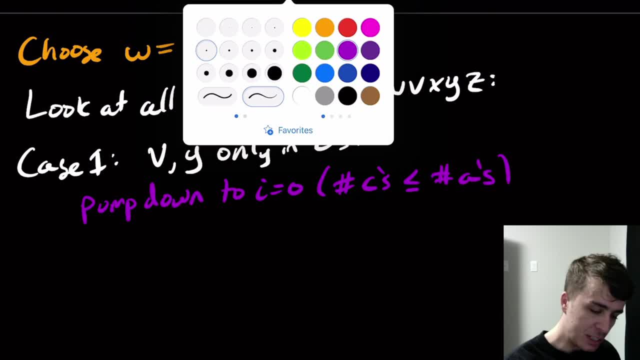 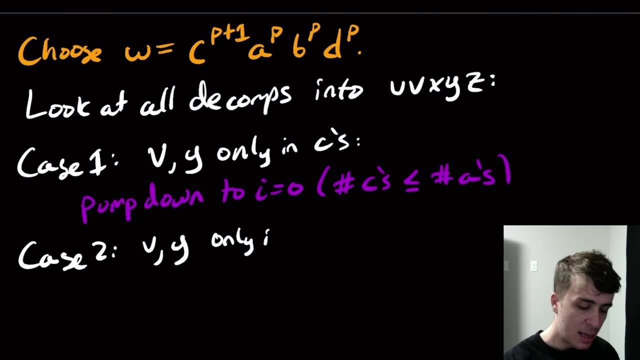 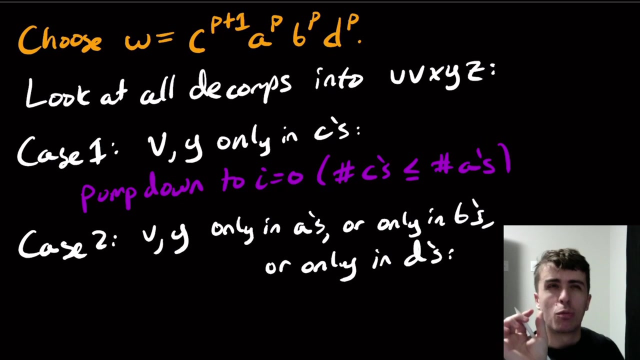 other. so if we have a second case here, we can actually group a lot of things, possibilities, together. v and y are only in a's or only in b's or only in the d's, and so it's only- uh, we call this a uniform in that it is only one character. it doesn't have two different characters. so in 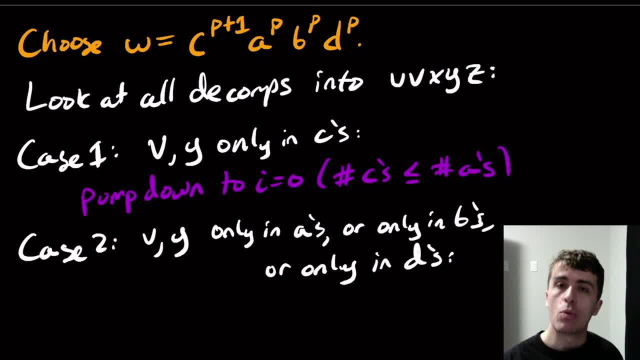 those cases. let's just say example for the a's. then we want to have more a's than c's, or at least as many a's. so if we pump up to i, equal to two. if we pump down then it won't work because we'll have fewer a's, but if we pump up we'll get at least as many. 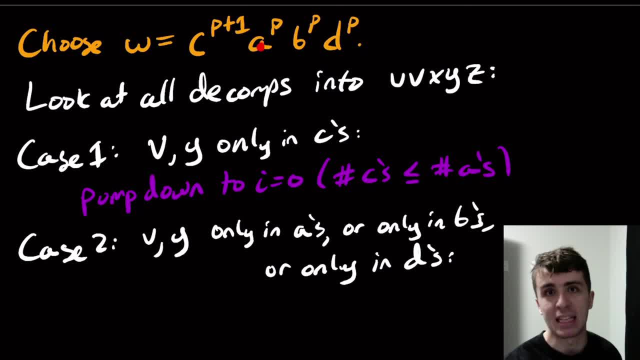 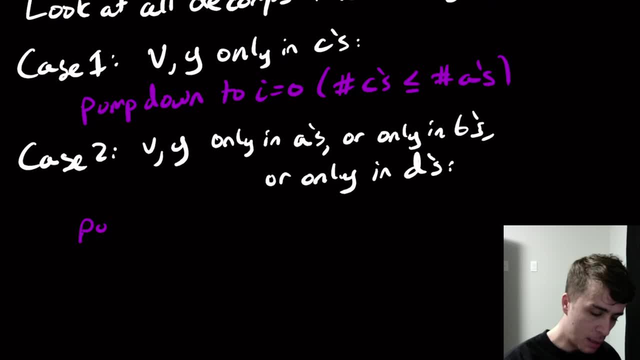 a's as c's, because we're obviously putting at least one uh a into the string. so, uh, what we'll do here is we will pump up the jam to i equal to two. so the number of a's, b's or c or d's- i have no idea which one it is, but it's one of those- will be at. 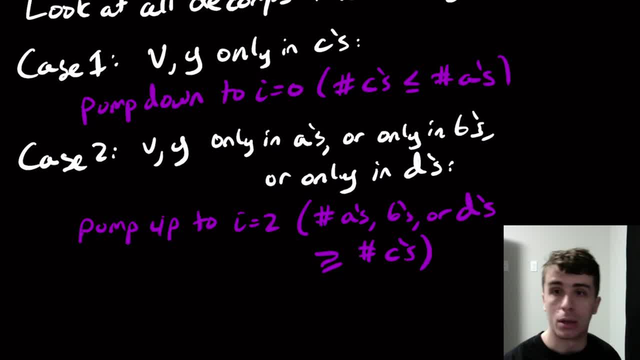 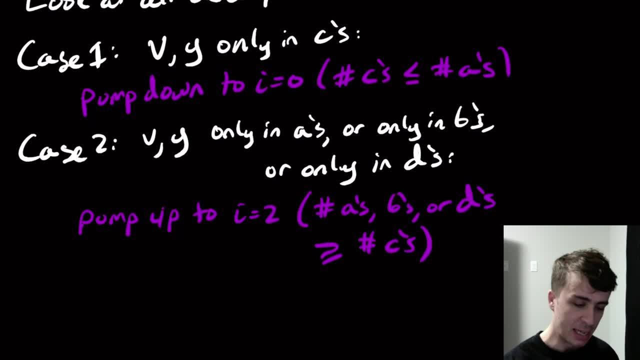 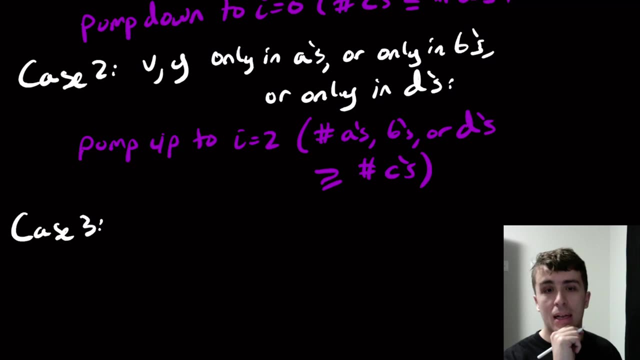 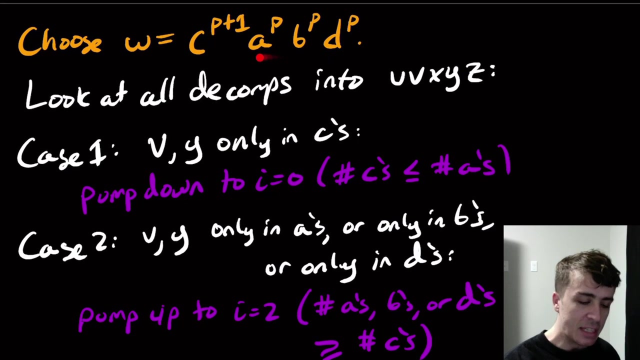 least the number of c's which will, which allows us to actually leave the language. okay, so now let's look at some of the more interesting cases. so, uh, so case three. so, uh, let's see, uh, if the v and the y part, it are only within this right half, this right half, like they. 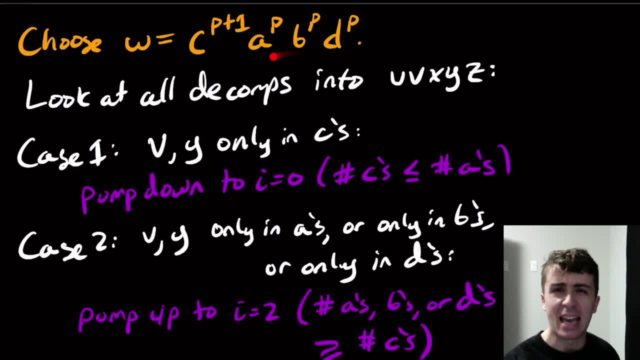 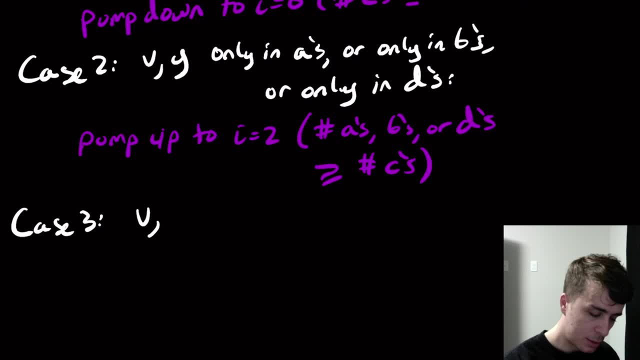 straddle the a's and the b's or the b's and the d's. it can't have all three for reasons we've discussed. so if it had a's or b's at the same time. so v and y only have a's and b's or b's and d's. 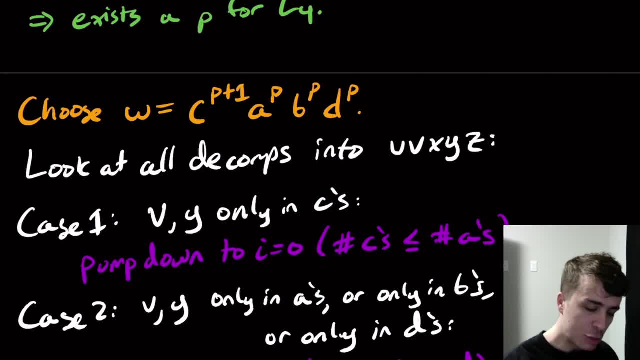 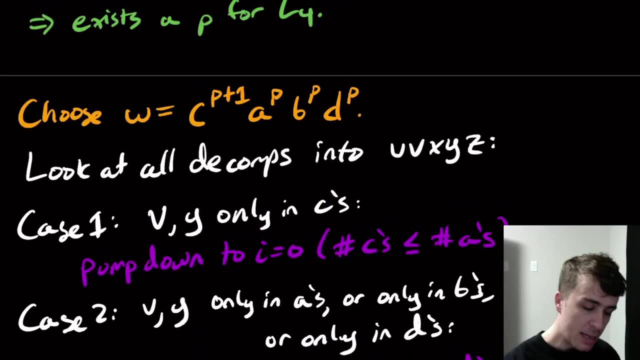 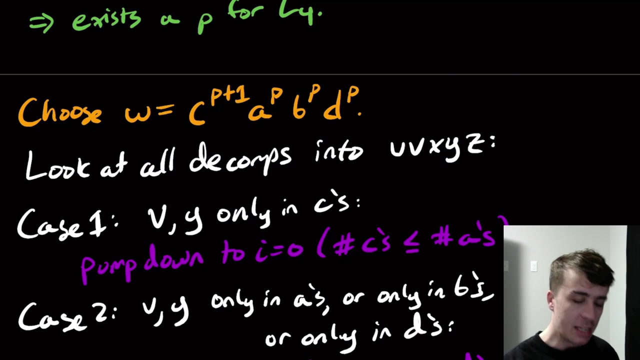 so it's saying that, uh, it's within this right half, but it has, um, it has, uh, uh, it's, it's between these, either between these two or between these two. so in either case, all a and b and d are symmetric to each other, so it doesn't actually matter. so what we'll do then is we'll just pump. 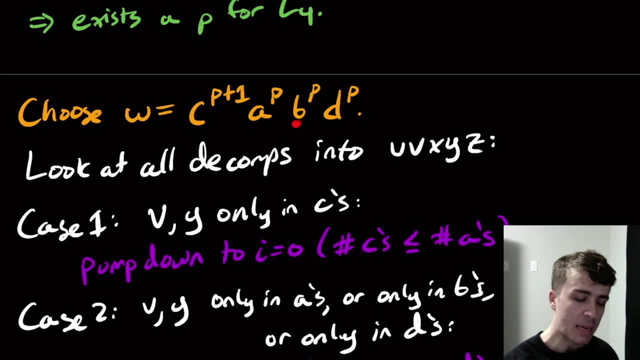 up just like before. i don't know which one will be inserted, but we'll just pump up the i equal to two, because i don't know whether v or y is empty. but i know that if if they're over here, then if i put more over to here, we're not having the number of c votes change. so the number of 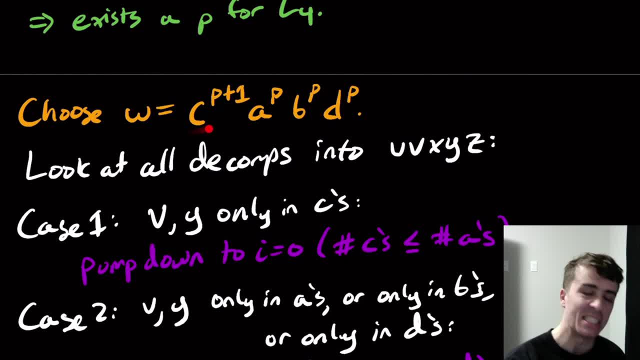 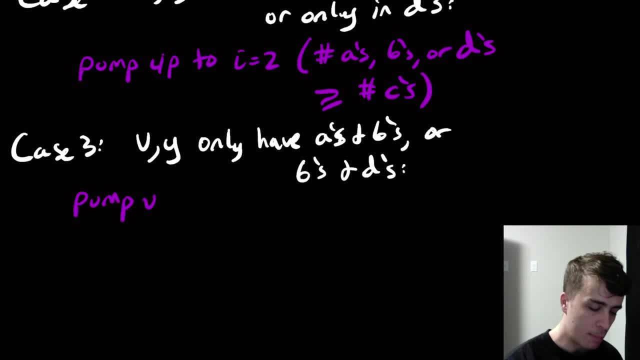 votes for one of the candidates over here will be at least as many as the number for c. so, uh, what we can do here is just like the last one: we can pump up to i equal to two, and so the number, and actually the conclusion is exactly the same. so we can pump up to i equal to two, and so the number. 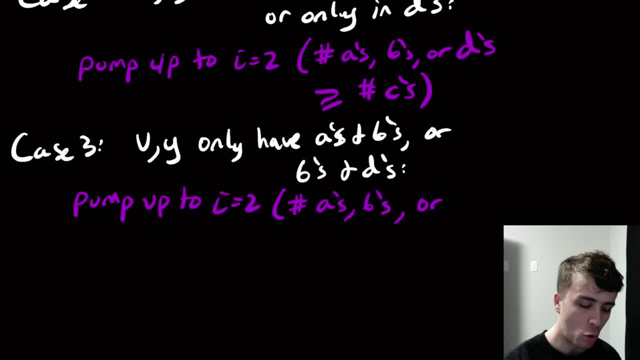 of b's- a a's, b's or d's- will be at least the number of c's, just like before. but uh, just like before, i don't know which one of the of one of them is the case. uh, it could be that two of them. 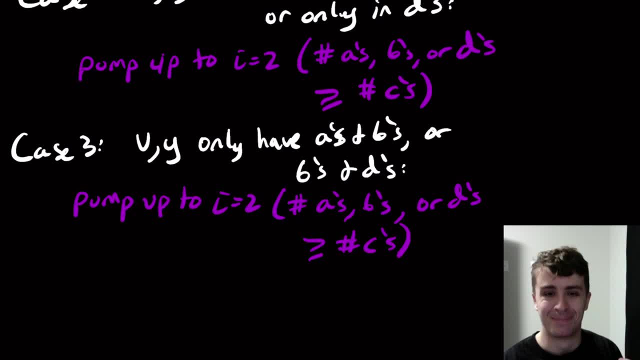 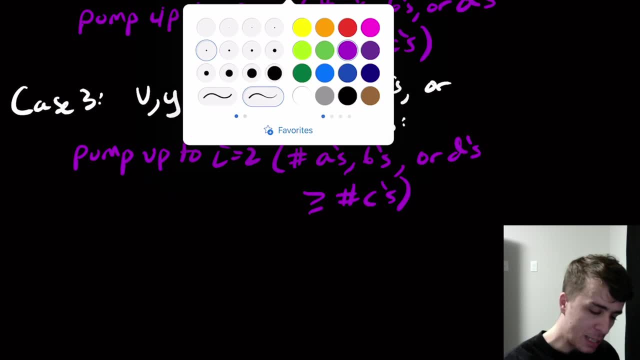 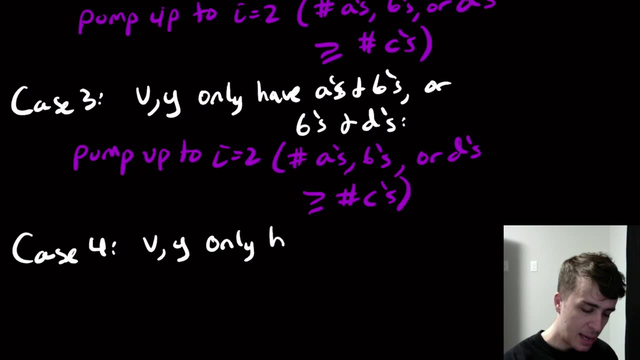 go up, but the important thing is that they beat c, okay. so so what do we actually uh do here? so the only other possibility, so case four, is that v and y only have c's and a's. okay, so they only have uh c's or a's and a's, and in fact, if it didn't hit, 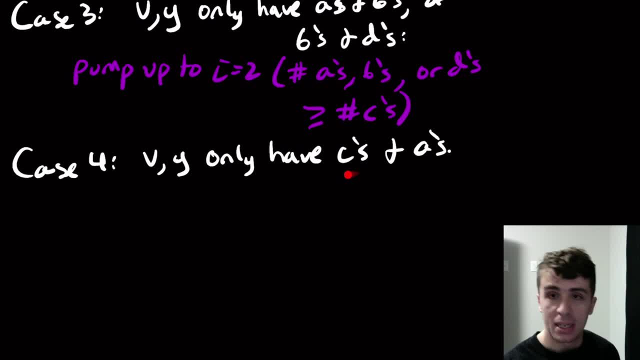 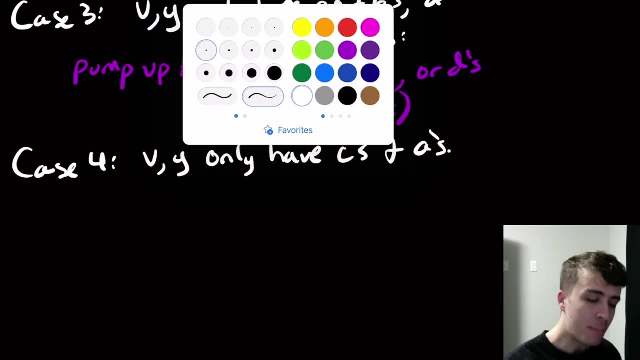 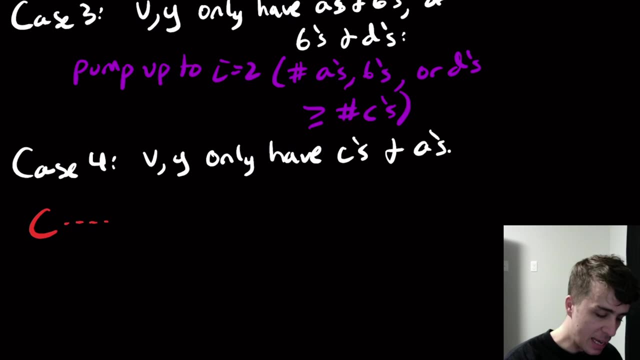 one of the other cases. we know that it must have at least one occurrence of c and one occurrence of a. so what will happen is what if we pumped down? so let's actually try to visualize this. so we have. we have c at the beginning, because that's how we design the string, then a's, then b's, then d's. so this is. 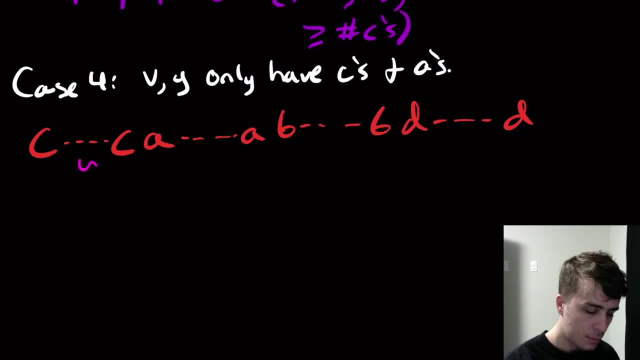 saying that the v part, which of course comes first, is in this, in the c's. but the y could have c's and a's. i don't really, it doesn't actually matter. so let's just say that it has only a's, but it could have um more. it could have some of the c's too. here's the, if we pump down. 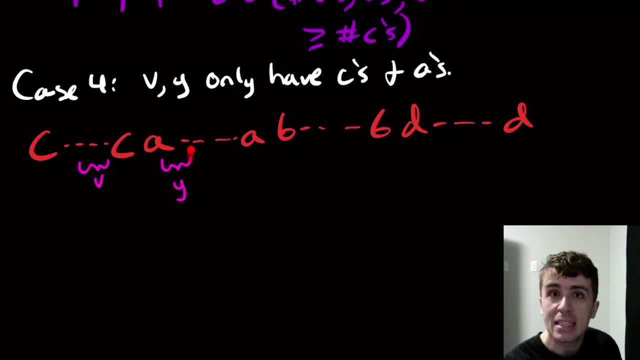 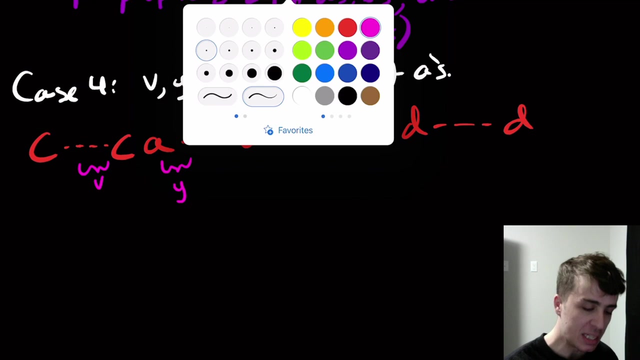 then, And it could be that the number of C's and A's goes down, but we don't know which one for sure. But the key is, the number of B's and D's doesn't change, And so, because of that, one of these two will have more votes than C does, because we're taking at least one C away, which means that the number of B's and D's will be at least as many as the number of C's. 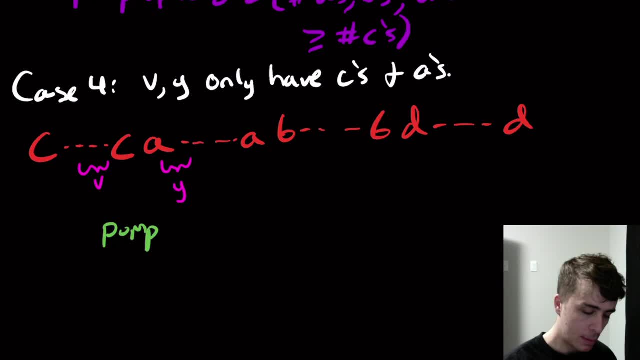 So in this case, if we pump down to I equal to zero, then what will happen? What will happen is either the number of B's is at least the number of C's, or the number of D's is at least. Oh, I forgot to put a number sign there. 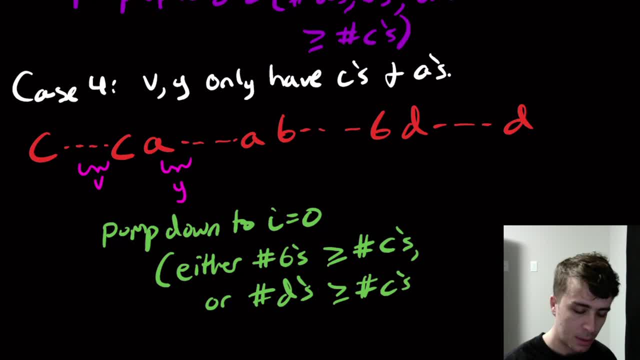 So number of C's, number of C's. One of those two occurs. I have absolutely no idea which one, but I know one of the two will occur, And so in this case, C did not win by plurality. One of B or D will, but I have no idea which one. 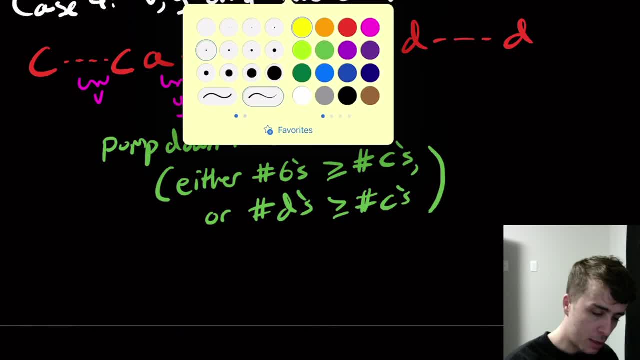 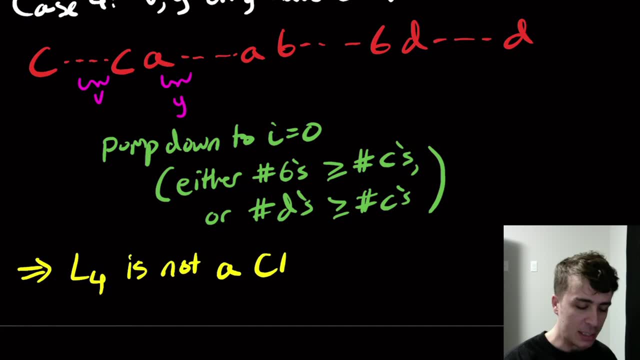 And so we leave the language in that case. So finally, after all that, we have finally shown that L4 is not a context-free language, because we left the language in every possible case. So hopefully that was interesting. Leave questions about the pumping lemma for context-free languages down in the comments. 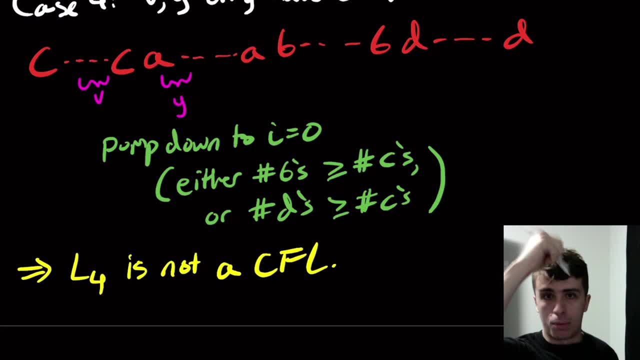 Or If you have any other interesting thoughts or problems about context-free languages and the pumping lemma down below. as always, please like and subscribe to the channel. It really helps us out. There are many other links in the video description if you want to support this channel further. And, as always, I'll see you next time.